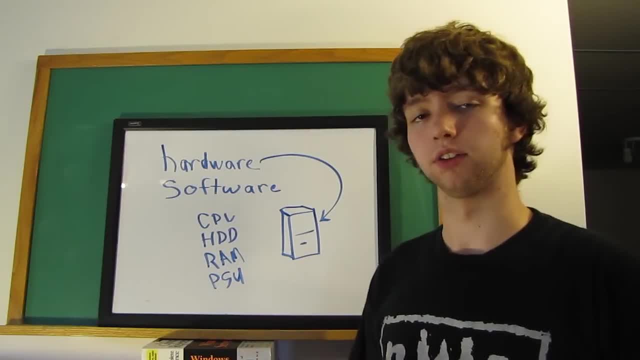 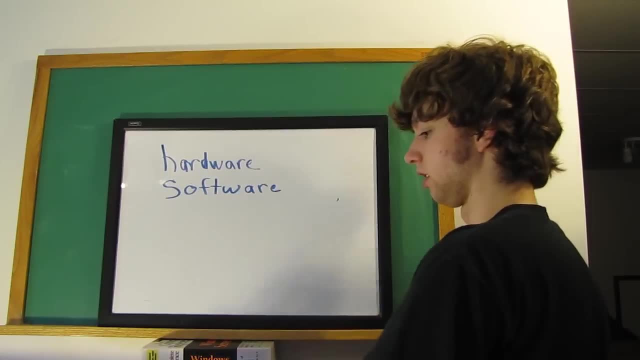 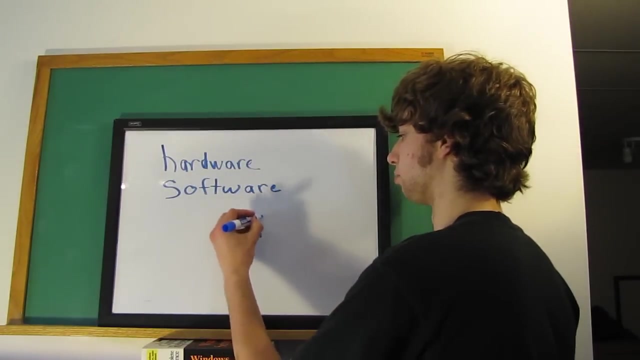 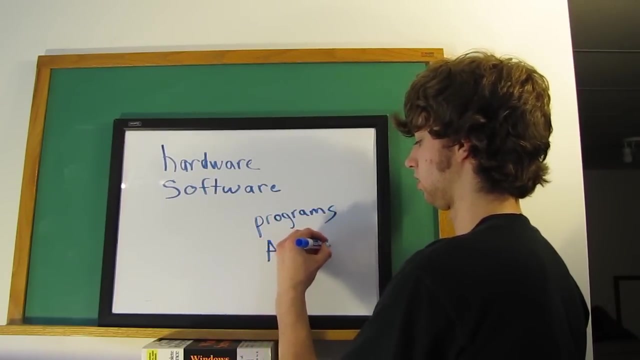 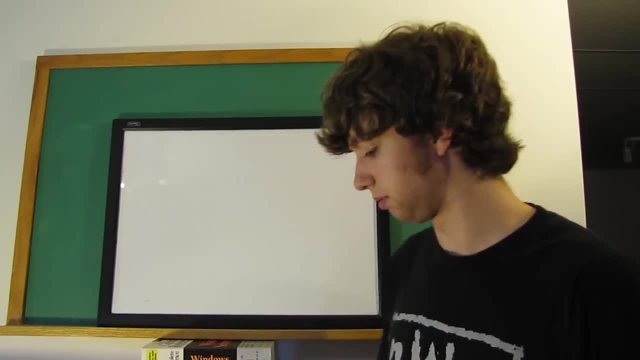 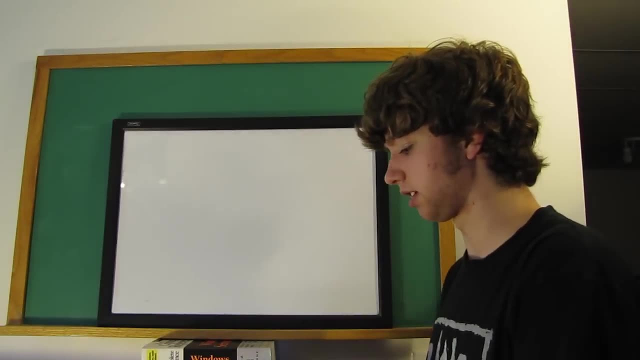 So, for example, web browsers So Firefox, Google, Internet Explorer Opioid. So, for example, web browsers So Firefox, Google, Internet Explorer Opioid. So an operating system is pretty much an intermediary between the software and the hardware. 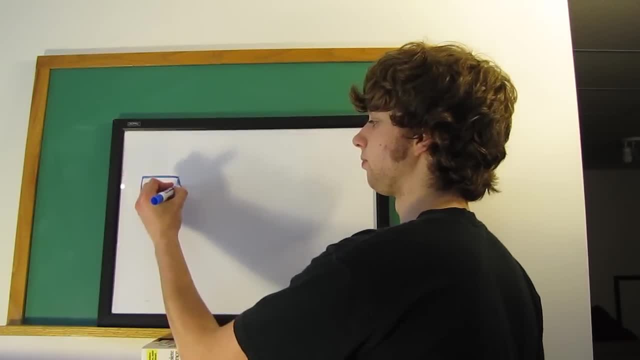 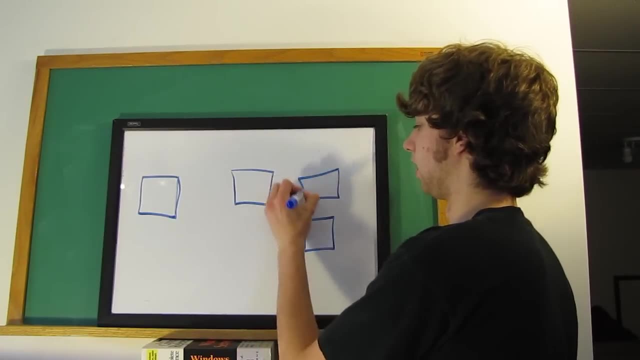 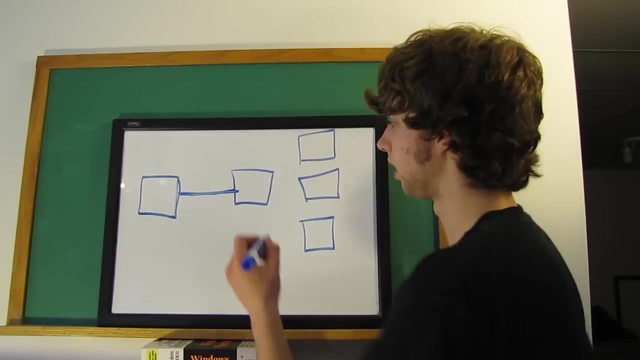 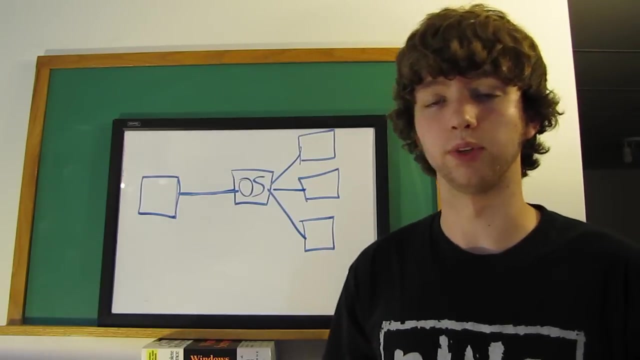 So if we have this software over here and then we have this operating system, and then we have three different types of hardware over here, Well, this software can communicate with the operating system, which then can communicate to the different computers. So now the person who's developing the app- 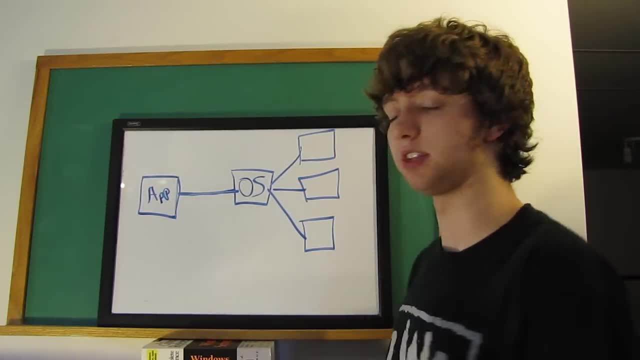 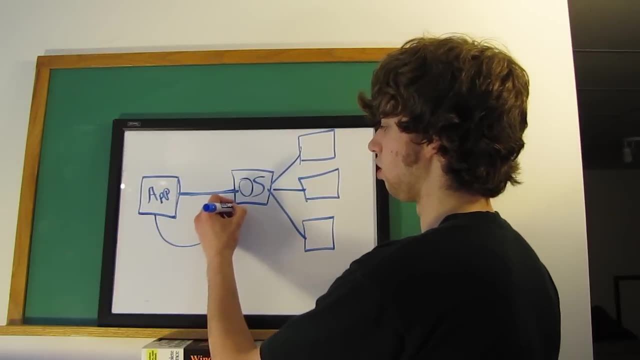 doesn't have to build it so it can do all of these things as taking information from the hardware and using it for its advantage. All it has to do is call on the operating system to do that stuff for it. Then the operating system does the appropriate job. 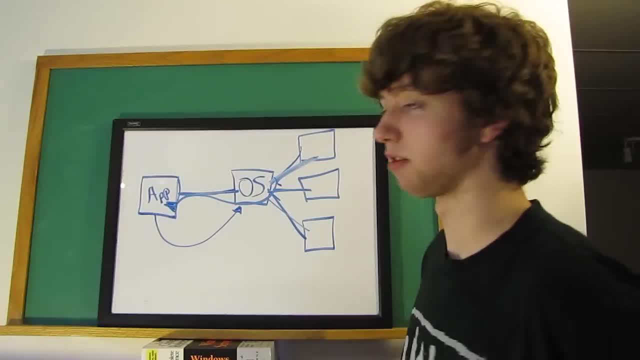 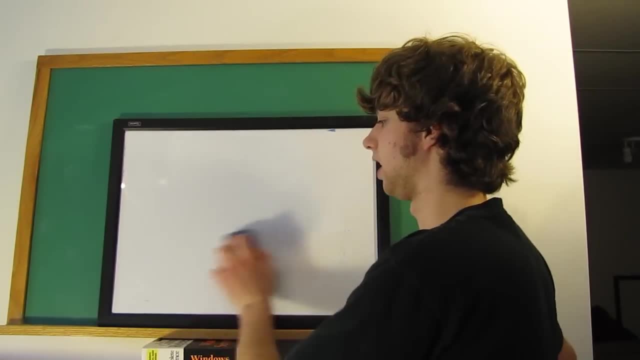 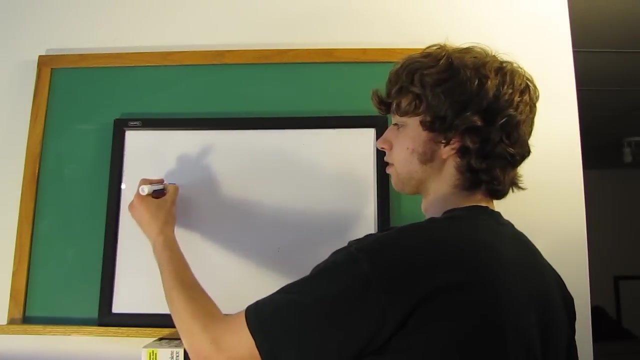 and gives it back to the application. So that is pretty much the process, Now the way things work together if we have an application. so I'm going to draw the application again, you know, because I always erase stuff and then redraw it for some reason. 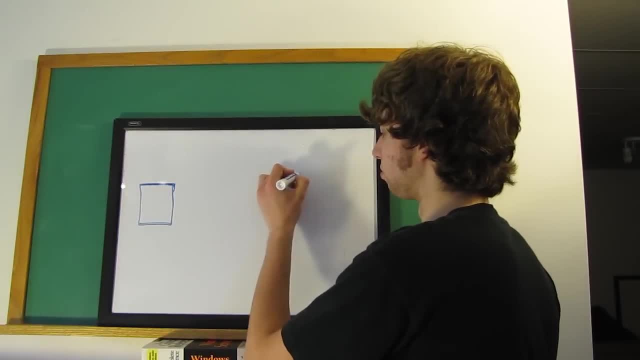 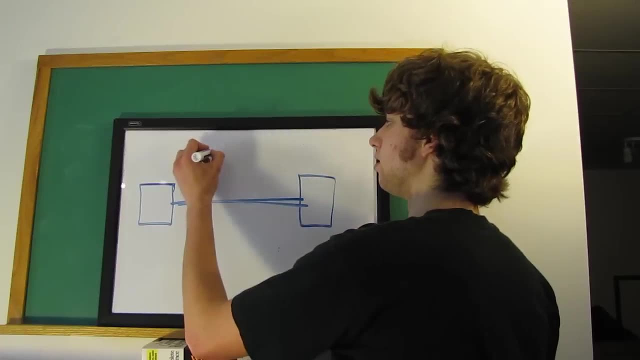 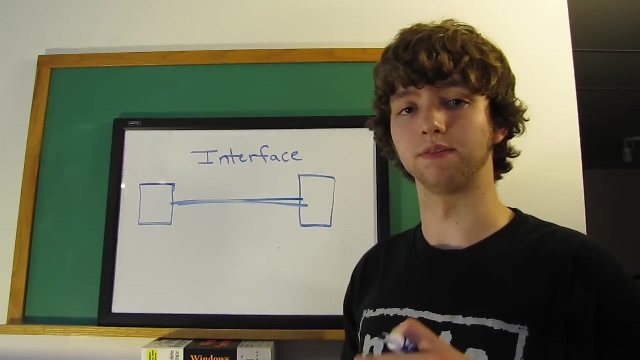 So here's the application and here's the operating system. So we're basically just zoomed in This means of communication. this is known as an interface. So basically, this is a system of standards and this allows the app. 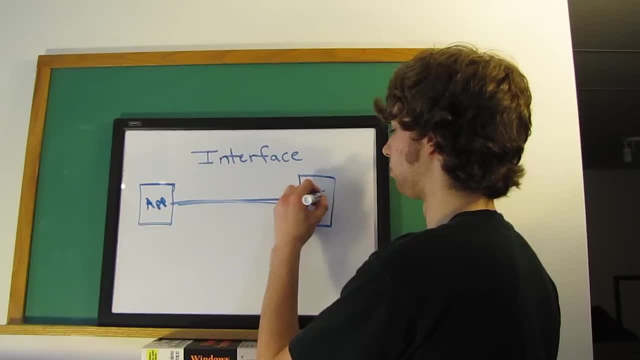 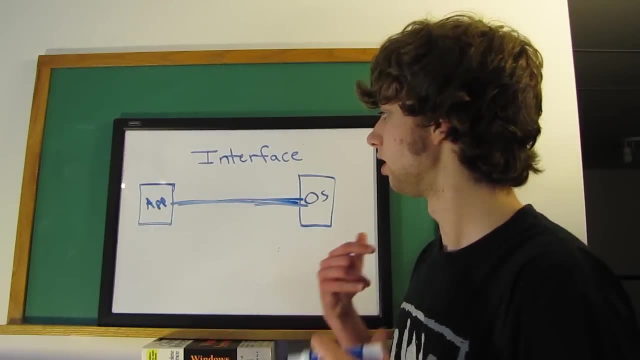 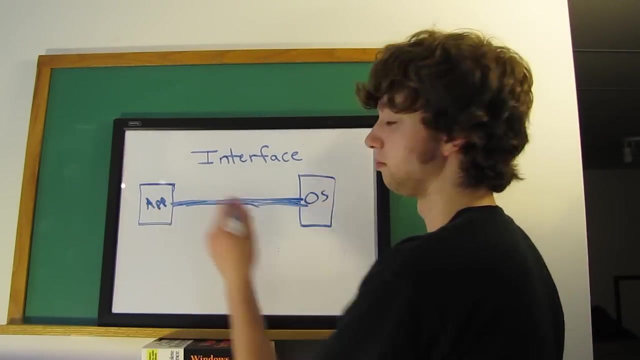 or the software to communicate with the operating system. So if these guys are talking basically in the same standardized language or whatever, then they can understand each other. So they follow a set of standards to communicate between between each other. 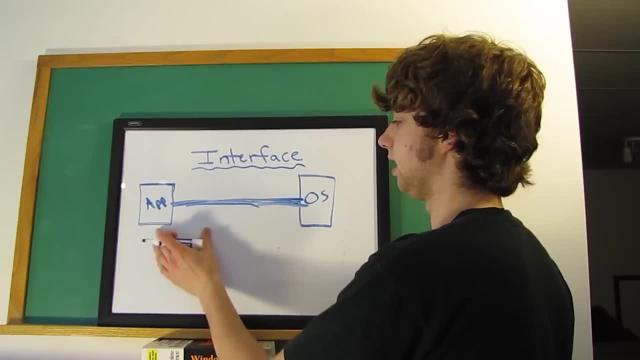 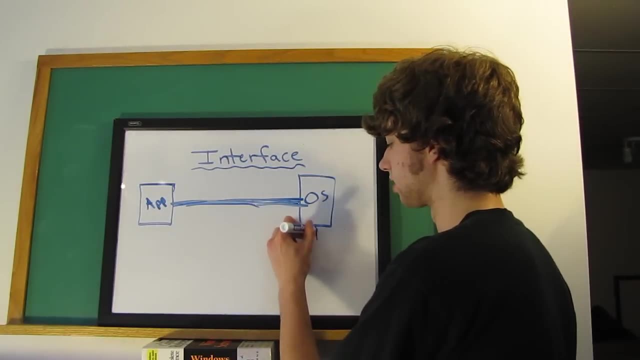 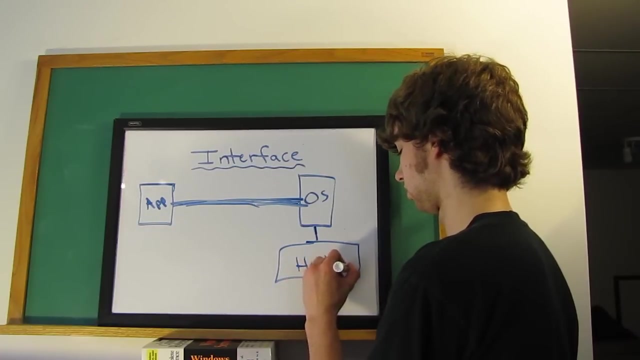 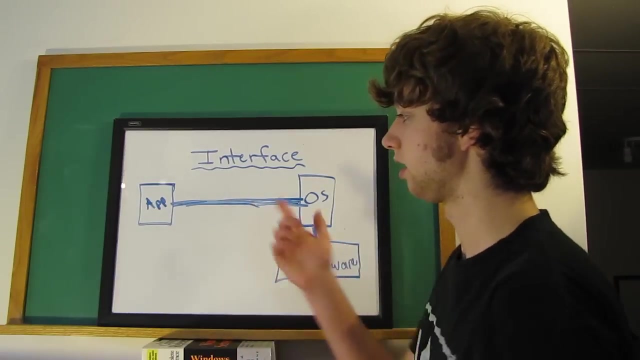 So this is known as an interface, and it allows these two to communicate. There's also an interface between the operating system and the hardware, So these are both examples of interfaces, Basically when they communicate. Now there's also another application. 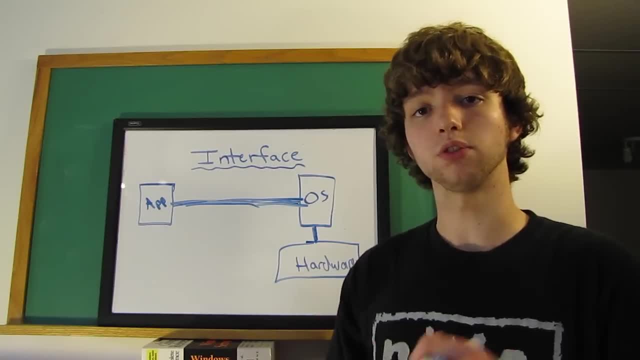 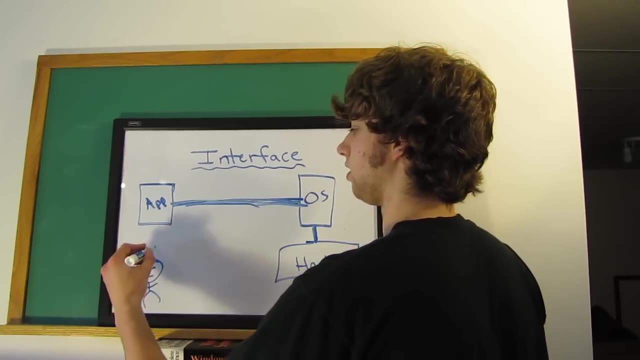 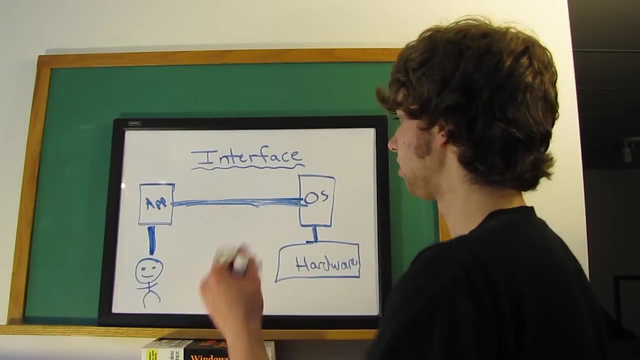 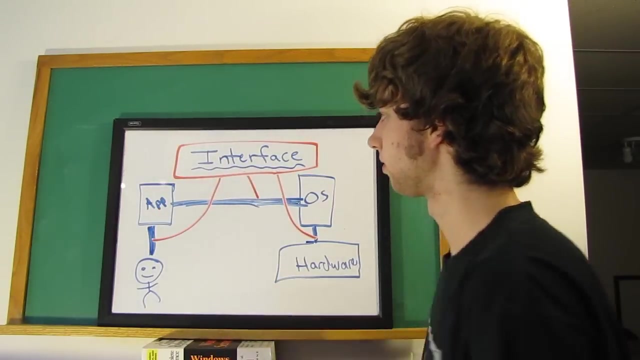 I mean interface. so when you're using your laptop, you could say you communicating with the application, this is also an interface. So these, these three means of communication, are all known as an interface. So with this system, all the application developer needs to know. 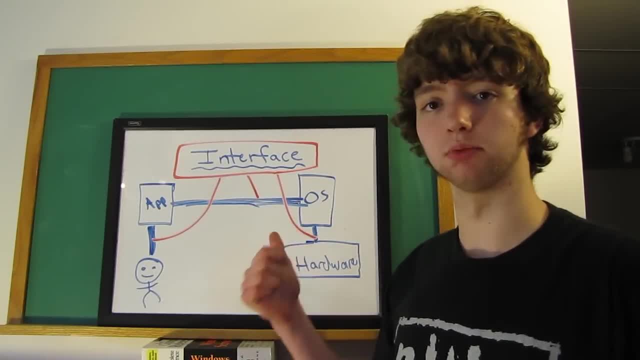 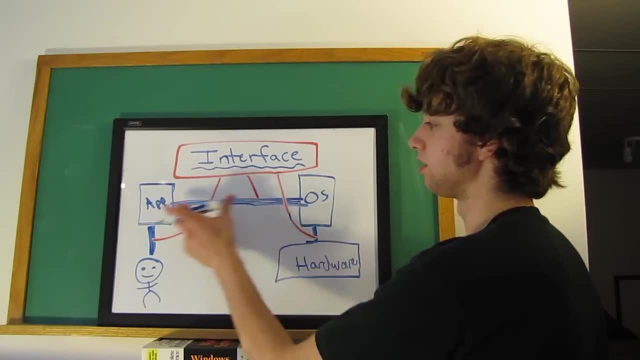 is what rules the operating system requires to communicate with the hardware. So, just like this interface, here there's specific rules that allow these two to communicate. Well, the operating system has specific rules to transfer that to to the hardware. 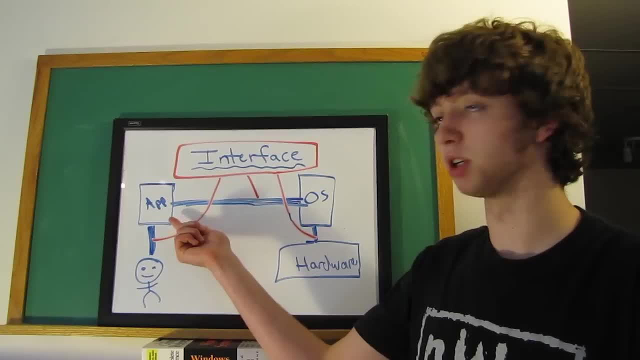 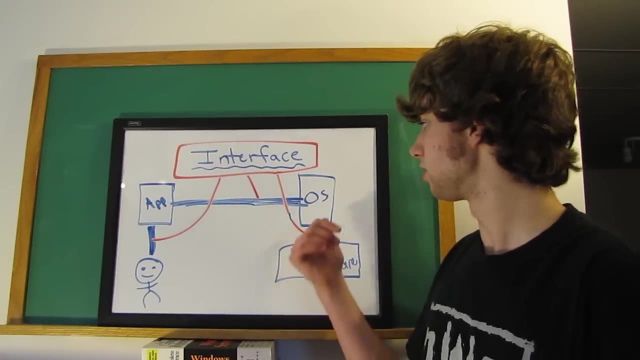 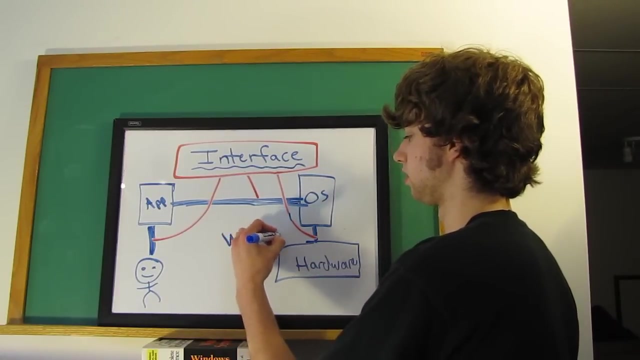 So this can allow the application developer to program a certain way to ask the operating system to do something with the hardware. So an operating system we could be using Windows 8,, for example, oopsies. well, Windows 8 has a method. 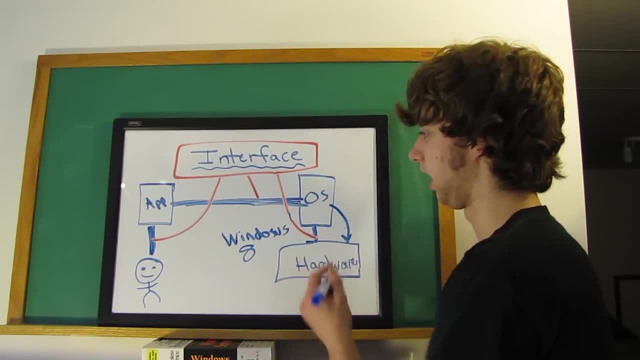 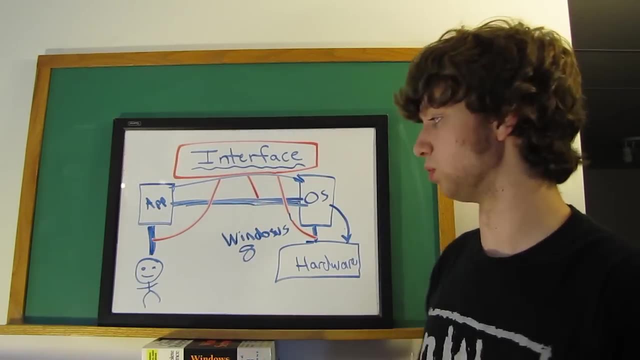 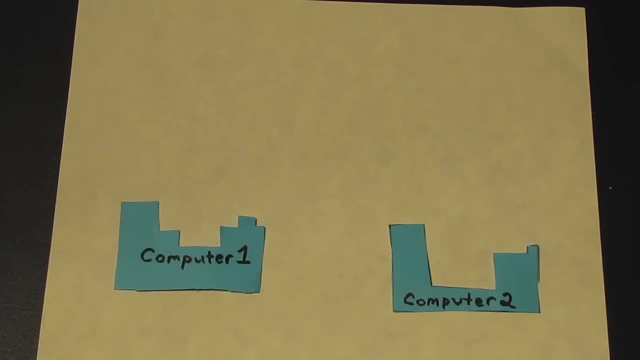 to communicate with the hardware And the application. within the code, it needs to tell the operating system to do that and the certain rules and laws that the operating system requires. Now to illustrate this concept visually rather than developing a professional PowerPoint. 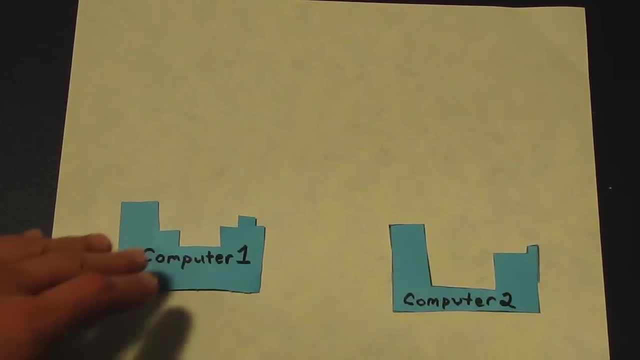 I just did some arts and crafts. So here we have two computers and I gave them different ledges to represent that they're different. So this one has different hardware than this one. They are not exactly the same. they're from different manufacturers. 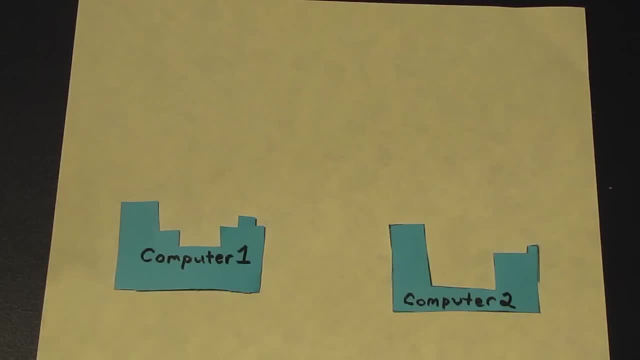 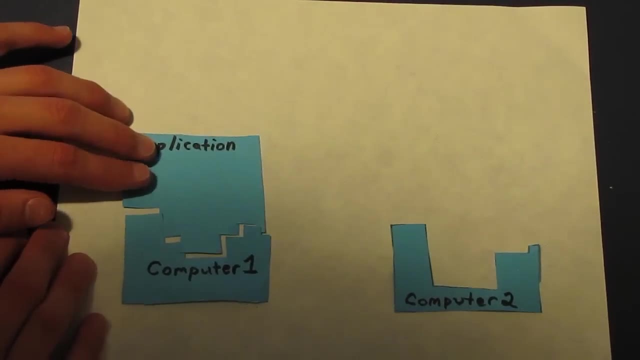 So now I build this super awesome application right here So you can see the application. Well, if you look, this is going to work with this computer here, cause they connect sorta. I mean, I am kinda bad at arts and crafts. 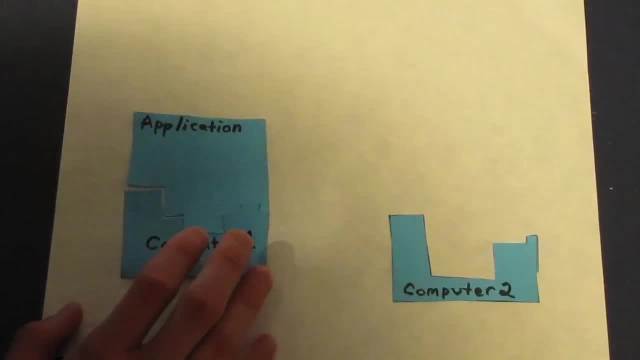 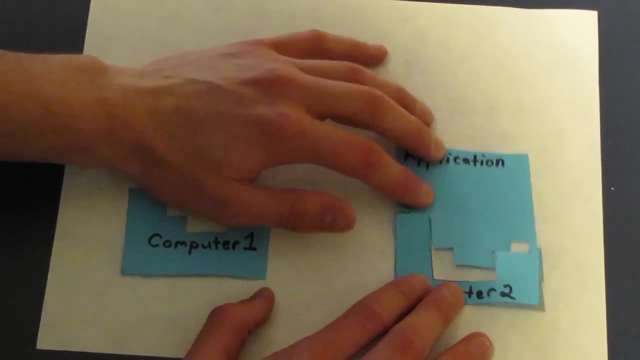 but yes, they do connect. Now, if I want to use this application on this other computer. well, you can see, it doesn't work out so well. there's some gaps and things aren't going to communicate properly. 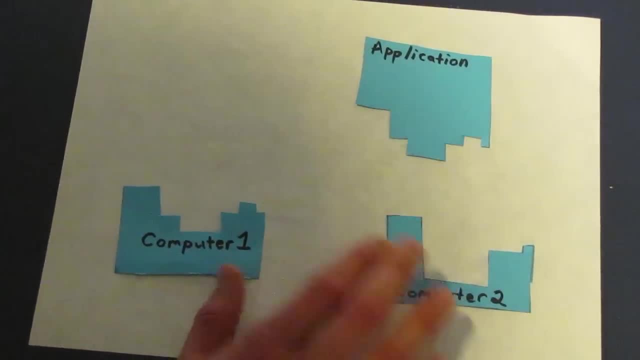 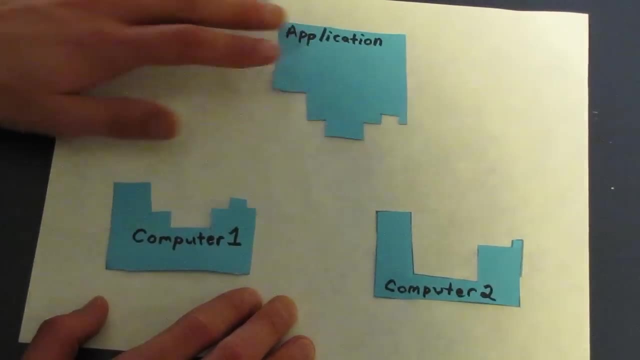 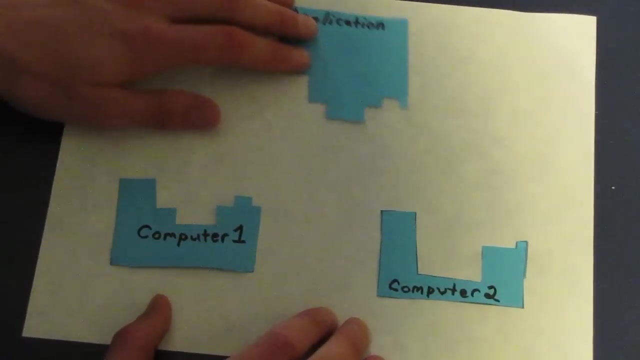 Well, these are two different manufacturers. now the application developer is given the responsibility to make it work for both computers, So they're going to have to allow people to submit their hardware settings and they're going to have to be able to reprogram. 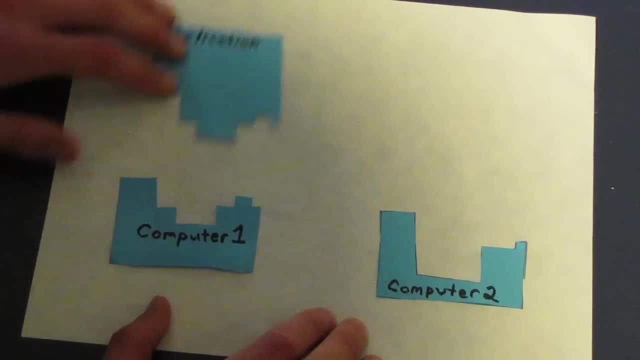 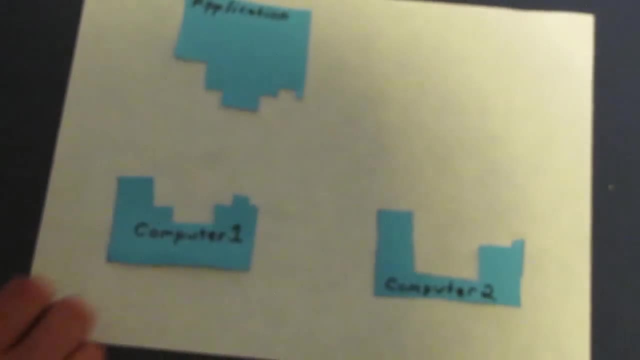 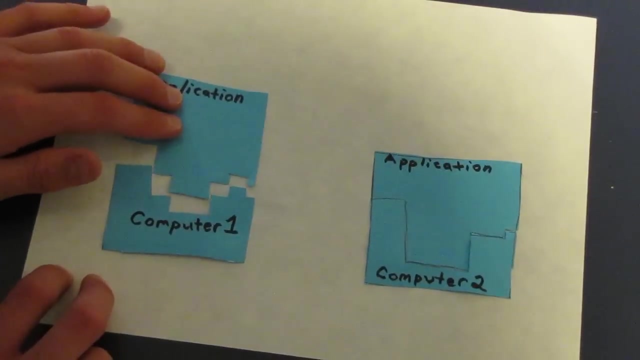 to where they can communicate with multiple different computers within the system, and you're basically going to get a modified version of the application. so this is the same application which can now communicate with this computer. So, as you can see, 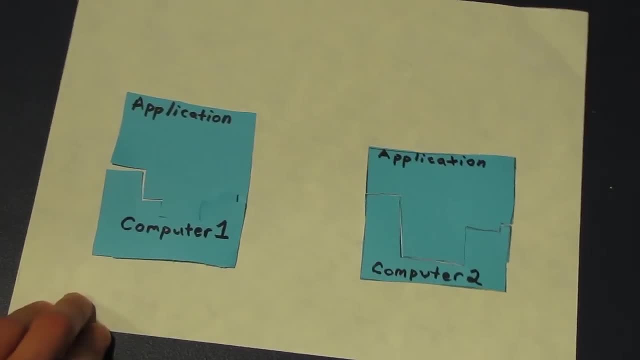 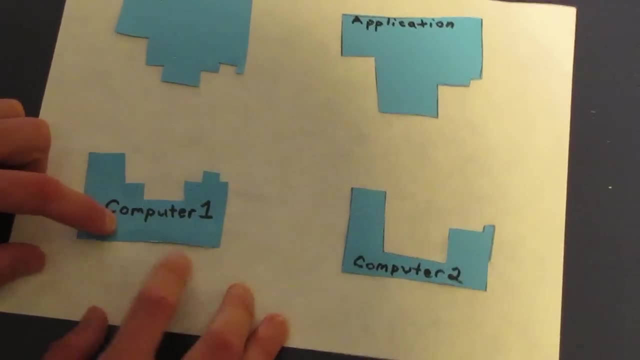 we can communicate with both of the computers, so that's good, although the problem is, the application developer had to develop an application that could speak with computer, one which is going to take a lot of work without the operating system. 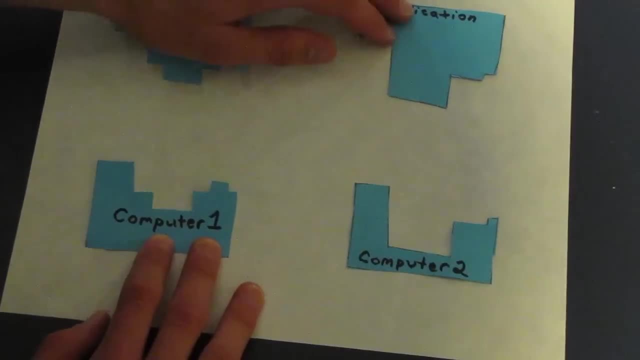 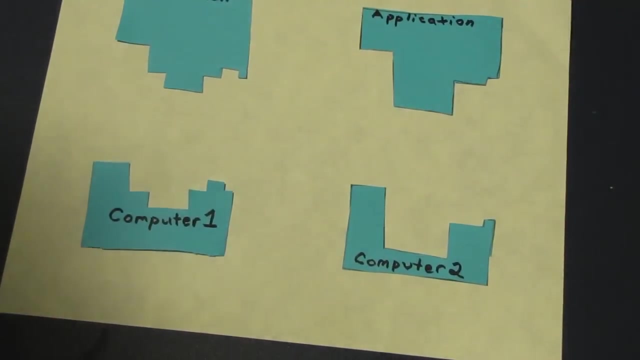 and they're also going to have to develop the same application that can work with computer two, not to mention many other computer systems. So that is the problem with applications without an operating system. to allow things to piece together easier. 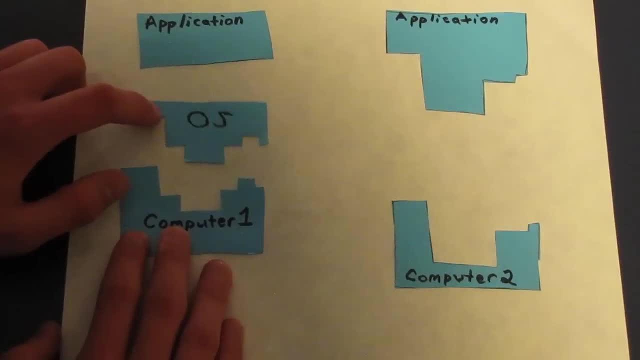 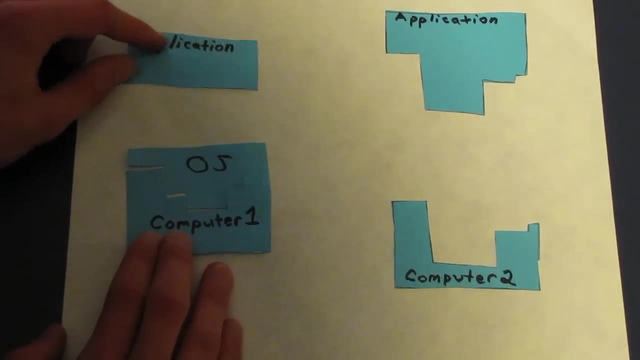 So now, what I want to show you is we have an operating system that can connect to the computer, which gives the application a platform to run on, So that not only we basically just took all the extra stuff. 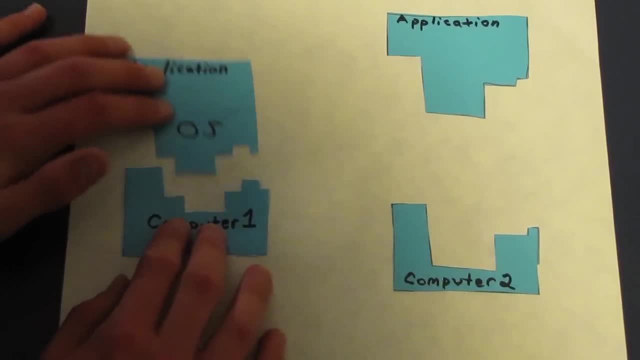 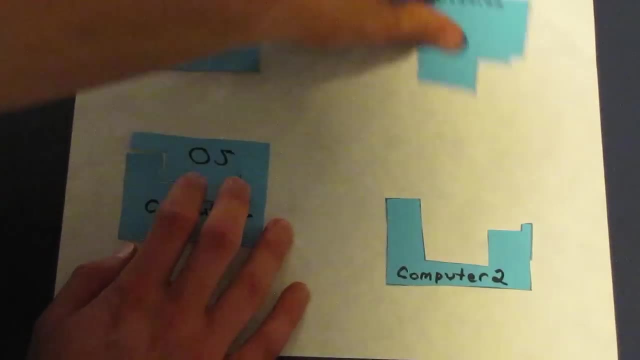 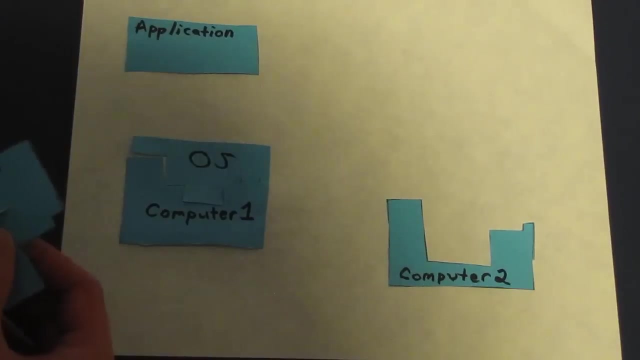 within the application that allowed us to communicate with the computer and we assign that to the operating system, Basically another piece in this process. So if we did this for this application over here, get rid of this extra stuff. so now we have an application. 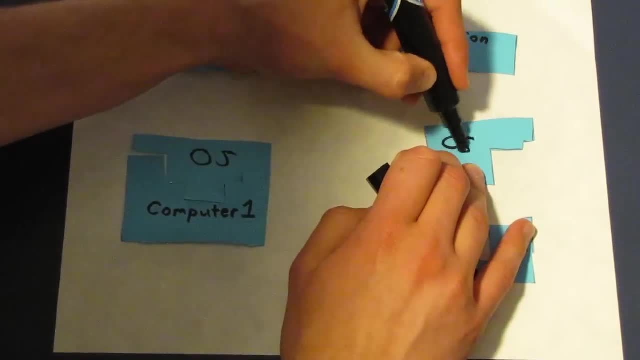 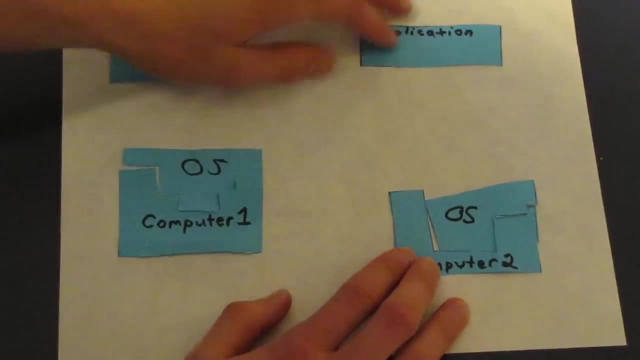 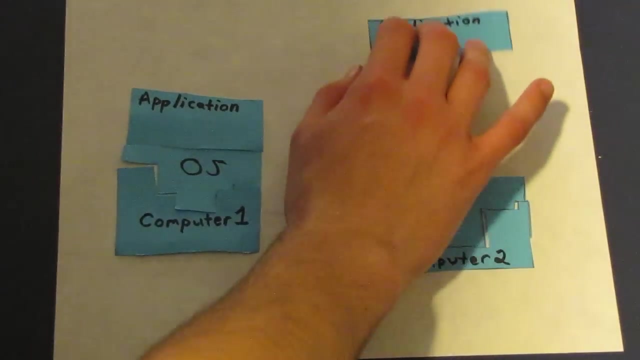 and we also have an operating system. So this operating system is designed to communicate with this computer, which allows a platform for the application to run on. So now we can run our computer systems. Well, why is this a good thing? 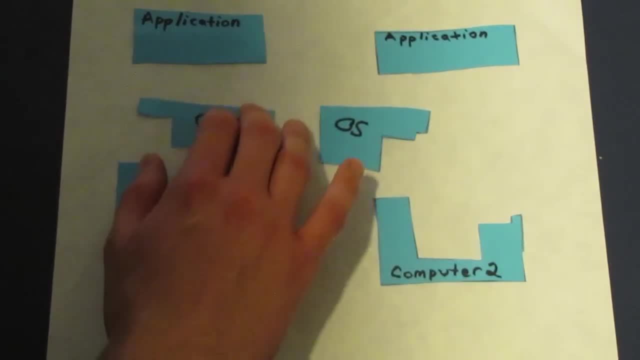 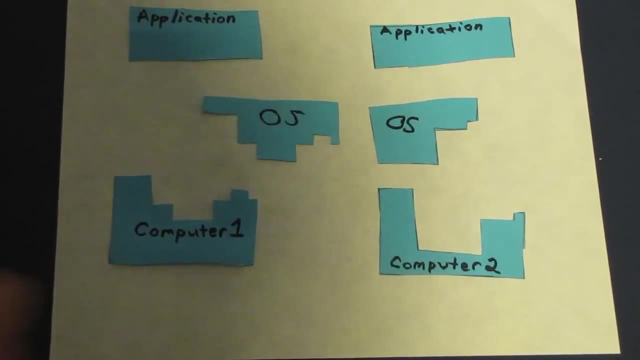 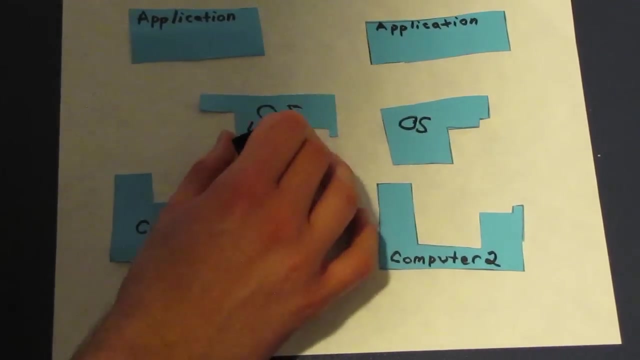 Well, first off, the operating system is designed to communicate with multiple forms of hardware, so this can be the same operating system. So let's say Linux, for example. This: this Linux operating system, is designed to work with computer one. 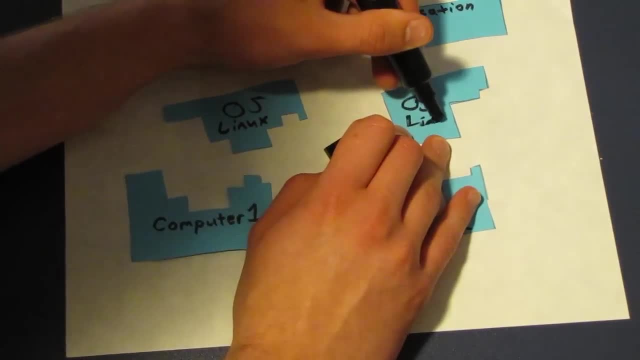 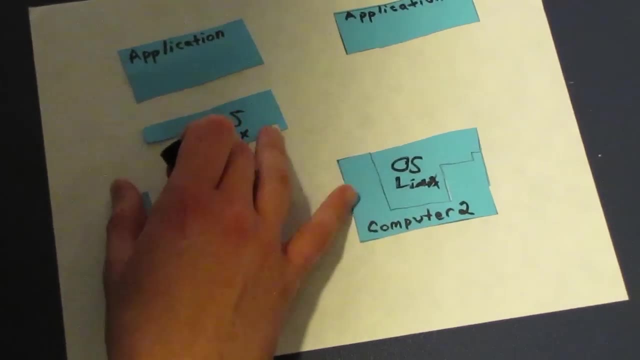 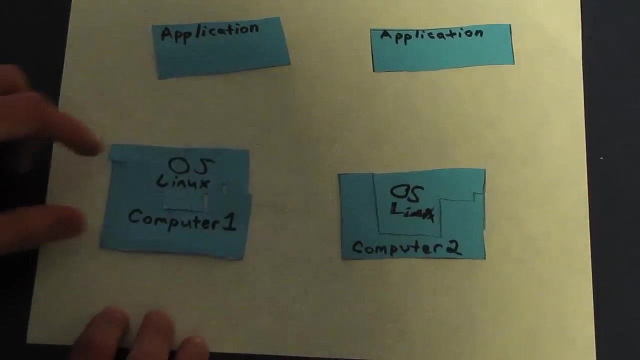 or it can work with computer two, So that's pretty much the operating system's job. It can do things such as request memory or allow multiple applications to run at the same time. So when the operating system 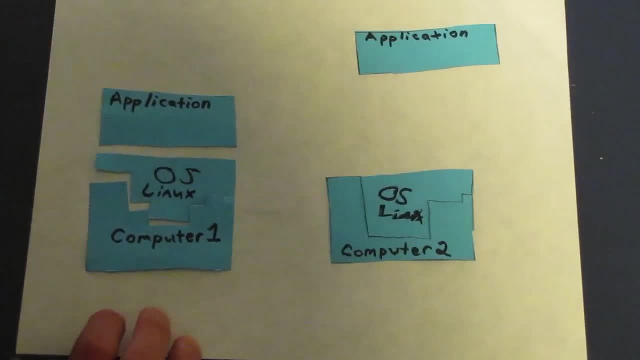 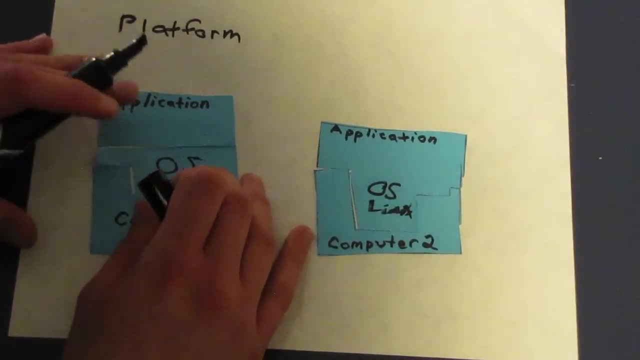 is connected to the hardware. we have what's called a platform for the application to run on. So now we can piece together our computers and we have a successful process here. So, for example, this platform is running. 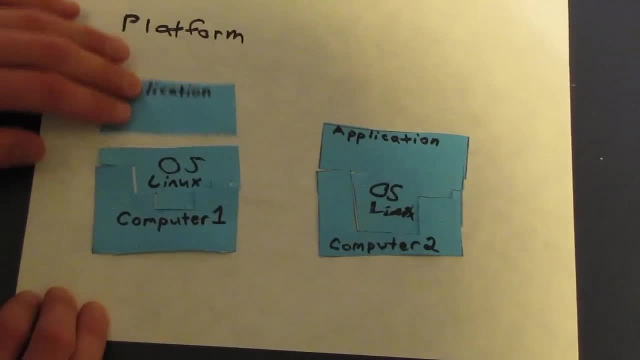 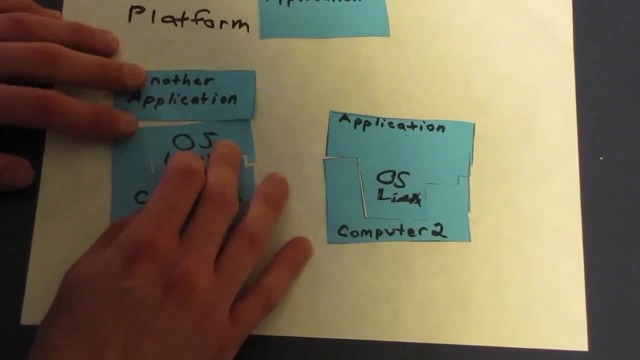 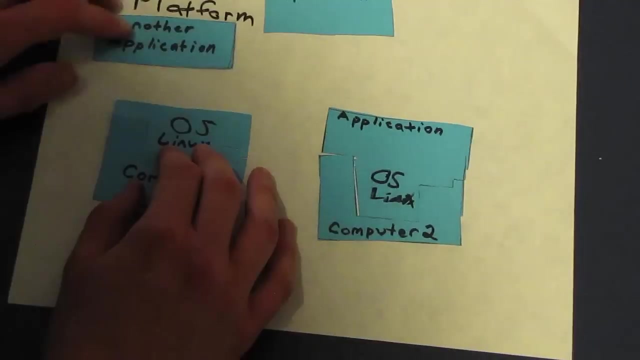 a Linux operating system. Well, Linux actually can understand another application, So these application developers don't even have to worry about communicating with the computer. All they have to do is worry about communicating with this nice platform. 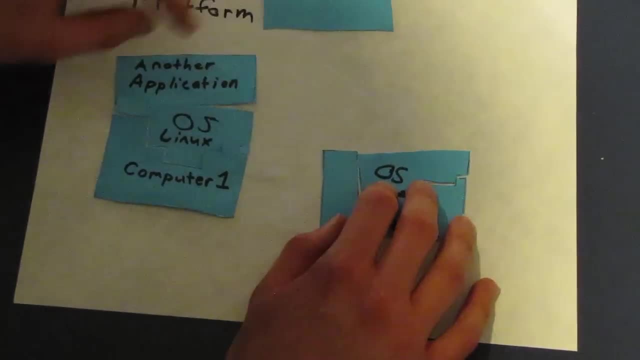 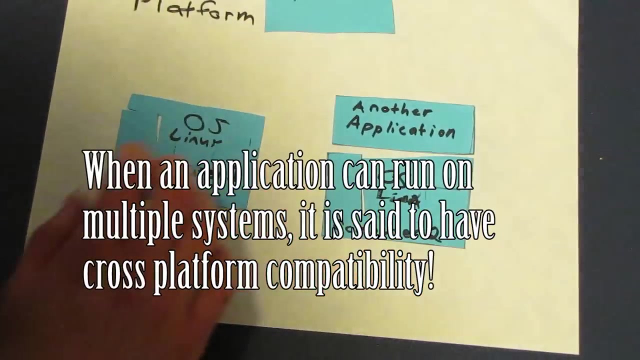 with the operating system And we can also run this on a different computer, for example. So now all of that work is sent to the operating system, which makes the application size smaller, because, if you remember, before it was like this big. 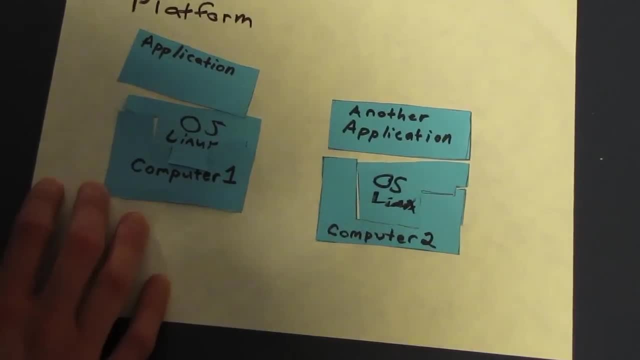 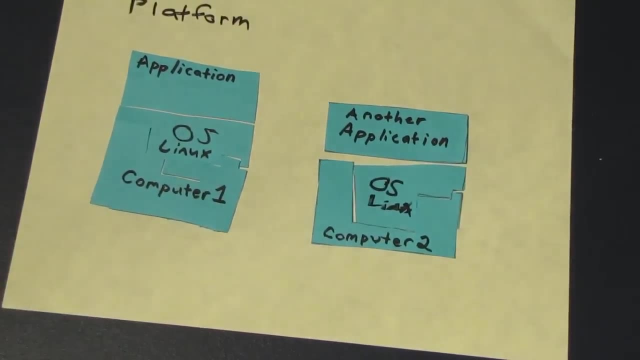 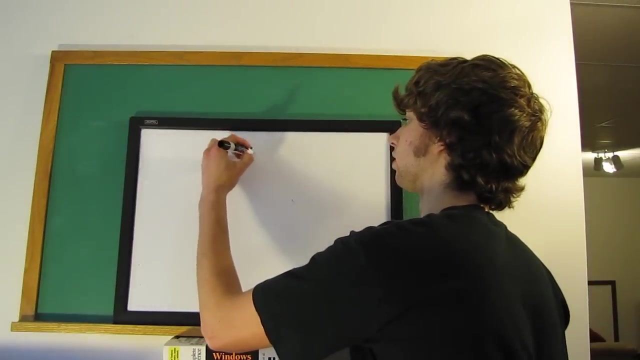 now it's only this big. So now the application is smaller and we don't have to work extra to communicate with the hardware. So from what we know so far, we have the user, the application or the software. 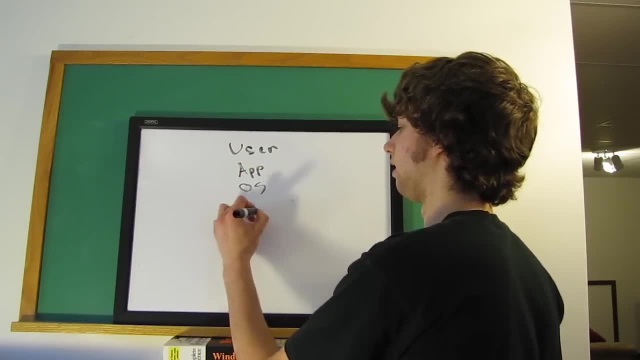 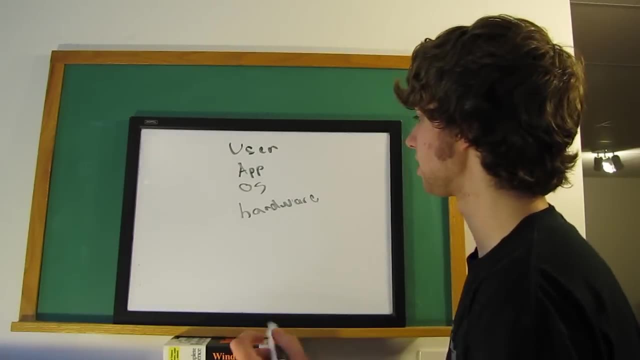 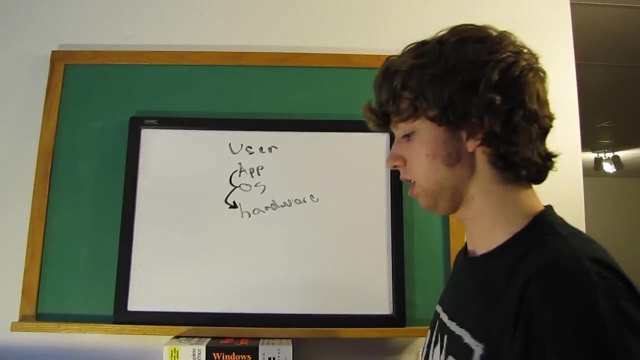 then we have the operating system and then we have the hardware, And I'm gonna get a bit of marker here. So, basically, the operating system allows the application to communicate with the hardware more easily. Correct, Well. 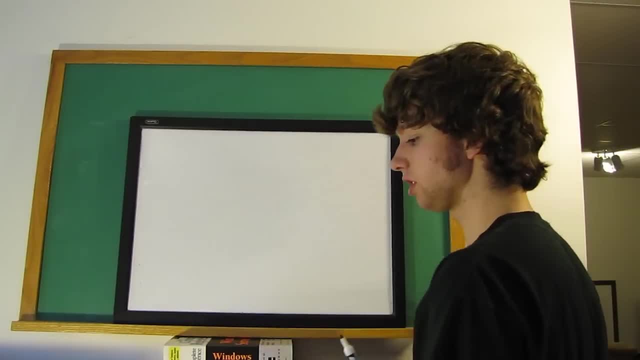 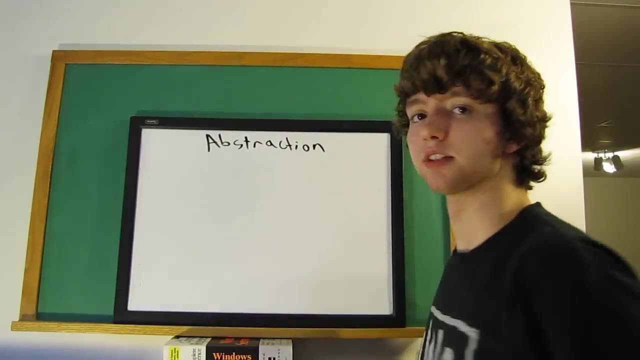 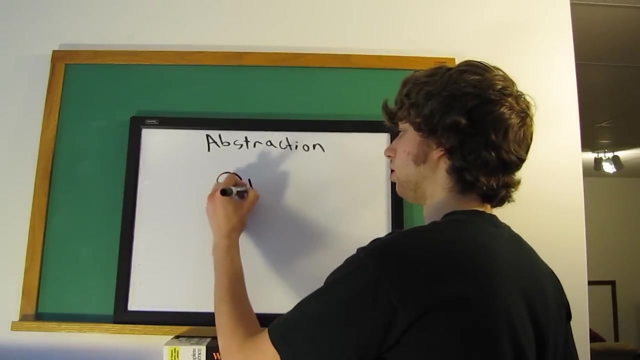 I wanted to get into something known as abstraction. So this is basically making something extremely complex and thinking of it in a simple way. So we think of it as operating system. We don't necessarily think. 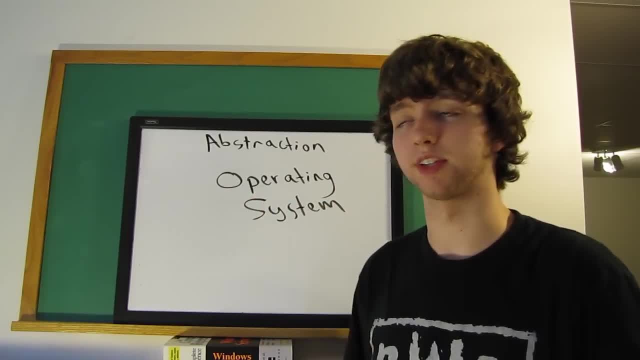 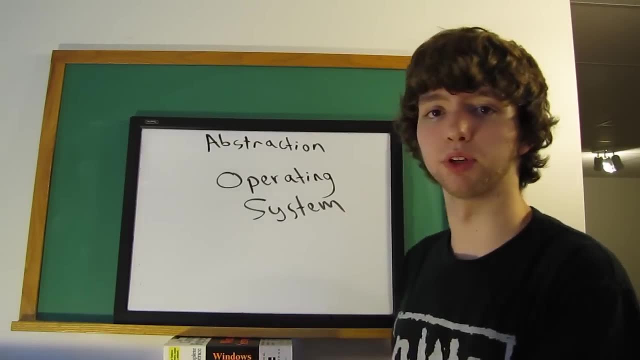 oh, the operating system has tons of services, has to worry about inputs and outputs, read and write requests. so if you save a file, it has to do something with. it has to communicate with all the different hardware pieces. 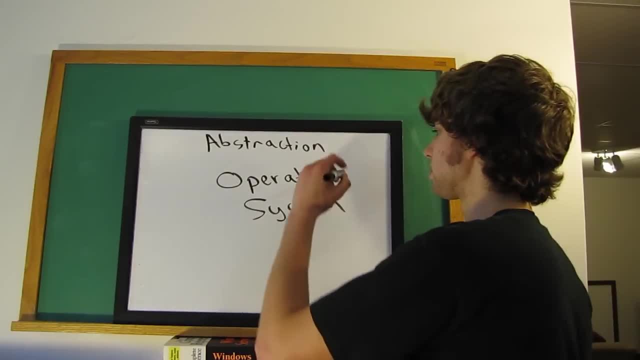 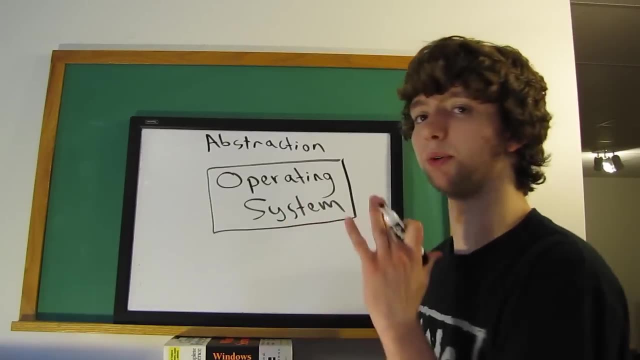 and blah, blah, blah blah and so forth and so forth. We just think of it as the operating system and we throw all of that work on the operating system and we don't necessarily have to think of the entire thing. 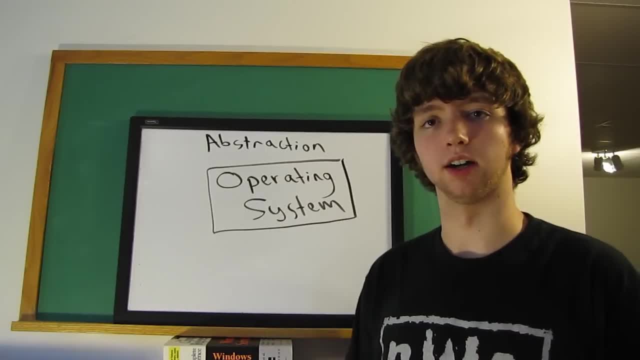 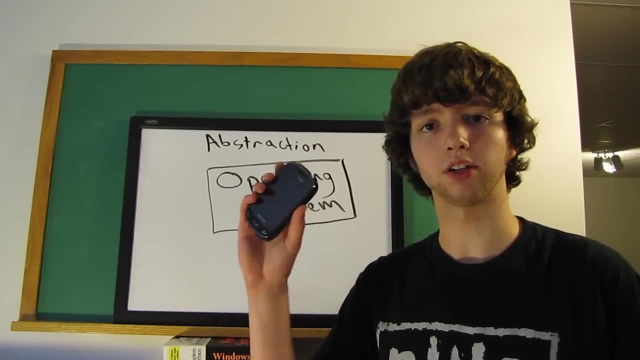 every single time we think of it. So that's kind of a hard to understand. So I got thought of an illustration. Well, here's a phone. If you know how to use a phone, you can type on it. 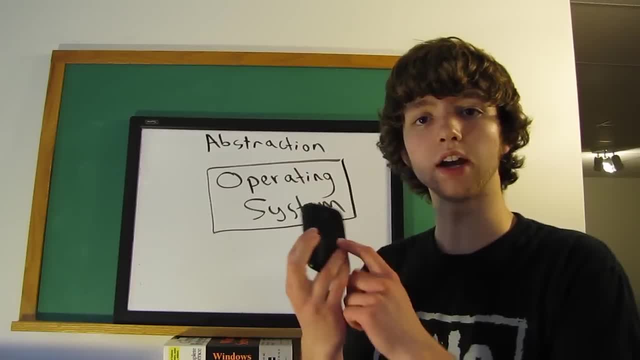 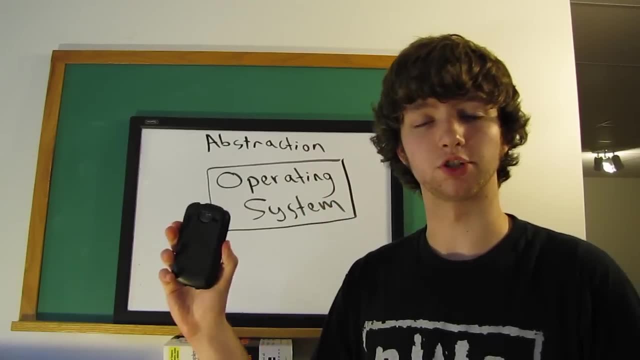 or call somebody, for example. Well, inside of the phone there's hardware and there's an operating system. so, just like, this is pretty much a miniature computer and once you figure out how to use a phone, 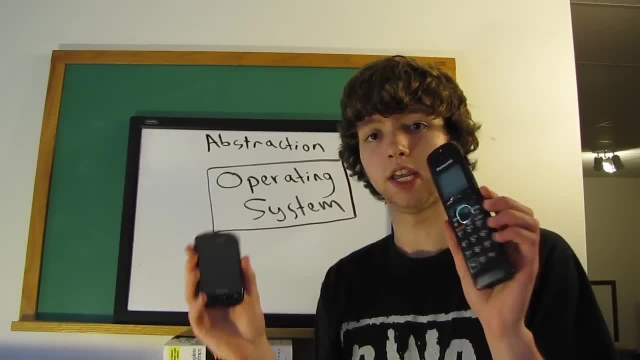 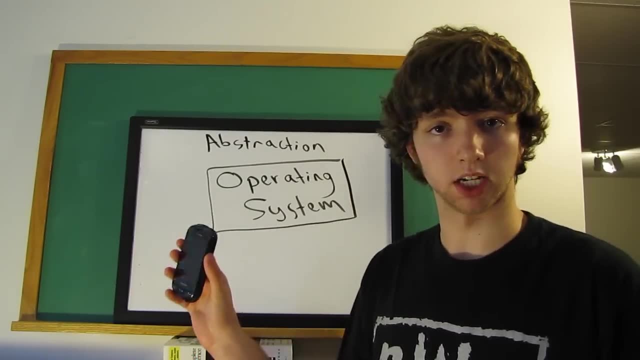 you can pick up a different phone and probably do the same thing. use it like this. So if someone's never used a phone before hand them a phone, it may take them a while to figure it out. 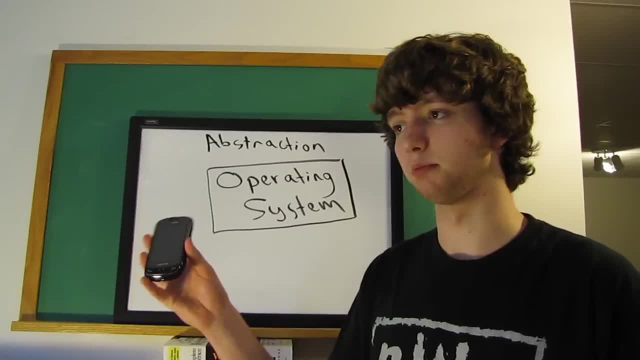 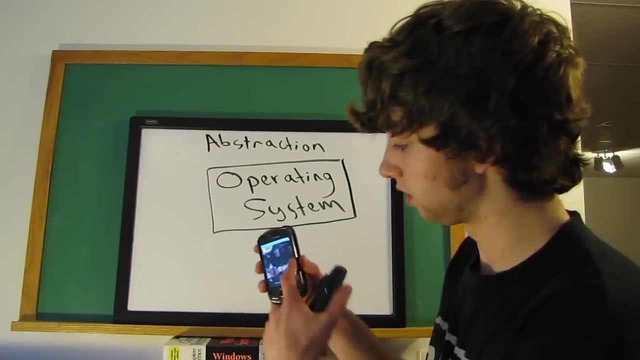 So this has an operating system, hardware, Symbian operating system, so forth, like that. But that's not always necessary to understand, because when you look at the phone, oh, you just press buttons, You don't have to worry. 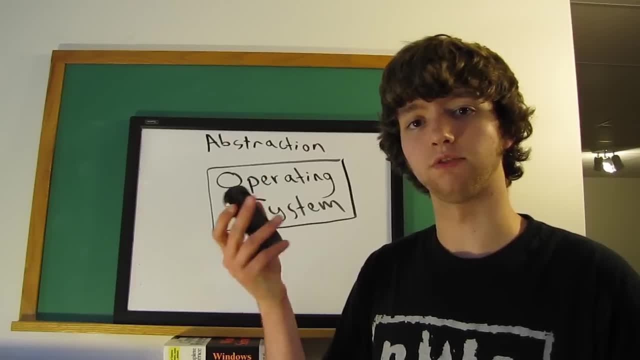 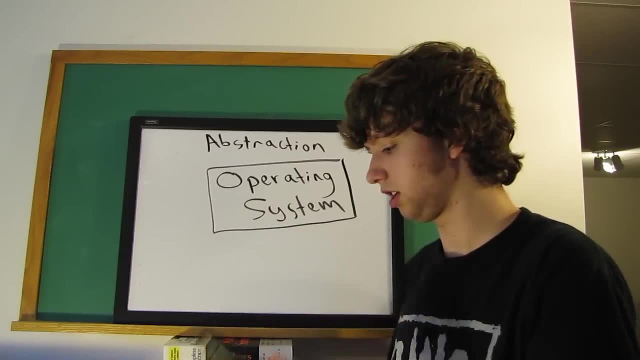 about the hardware within it. And then, once you figure that out, you can pick up different kinds of phones. So you can just pick up any kind of phone, talk on it. Hey, hey, what's up. 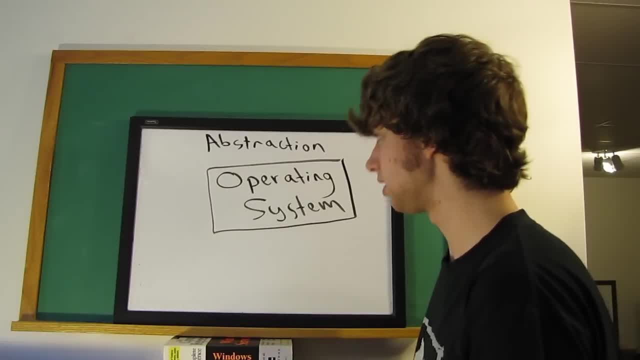 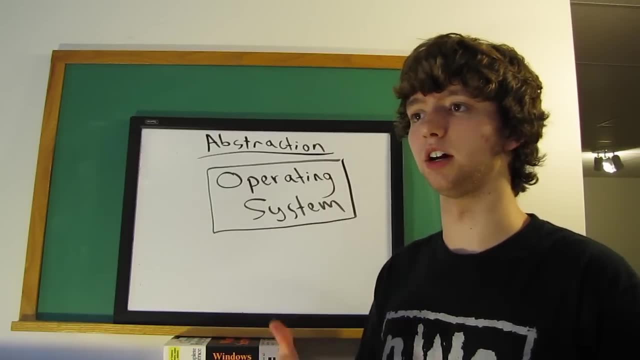 And they all kind of work the same. Well, this is an idea of abstraction. We're taking an abstract concept such as the entire phone sending the data to the other person's phone magically. Well, that's complex stuff. 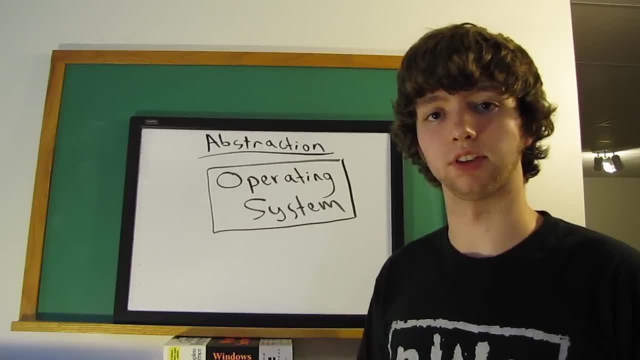 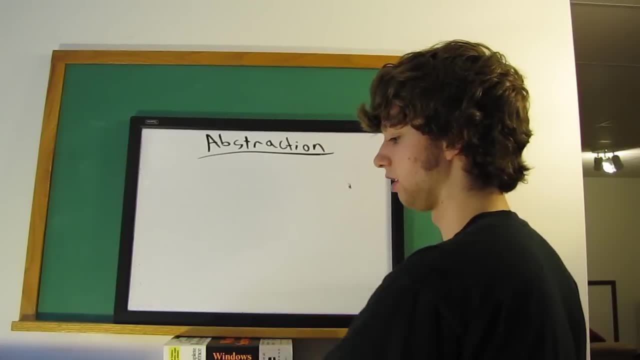 so we use an abstraction so where we don't have to think about that at all. So earlier I showed you like the setup. We had the hardware down here And then we had the operating system. 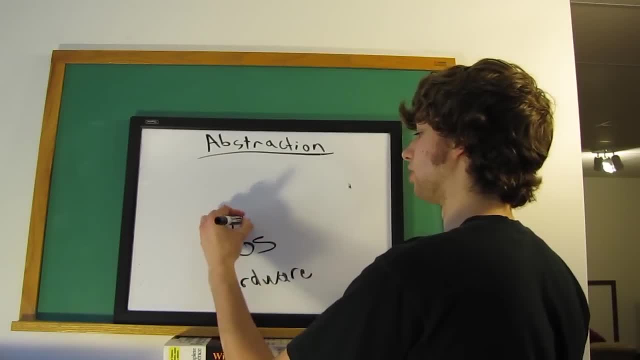 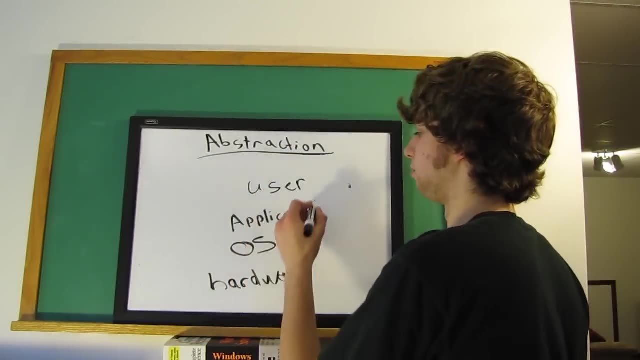 And then we had the application layer or the, the software, And then we had the user, And then between each one of these we had interfaces, Which is basically how they communicate, And then between each one. 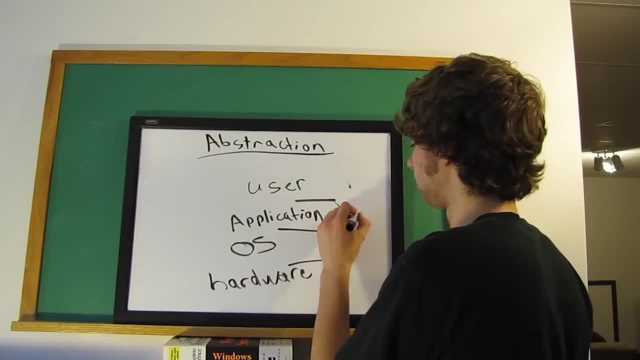 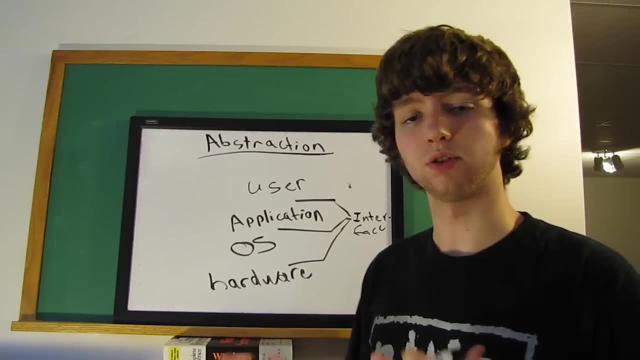 of these, we had interfaces. So this interface, All right. so this, this is known as layering, So layering And basically this allows us to think of this in an organized fashion. 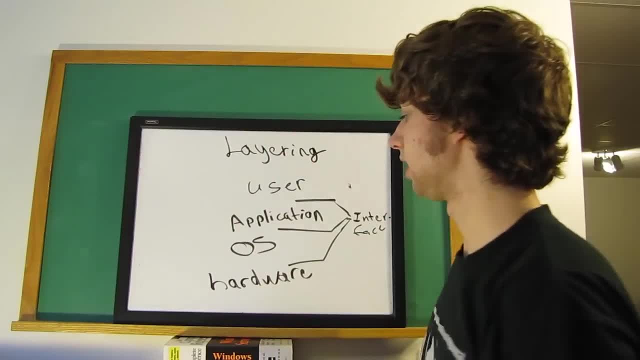 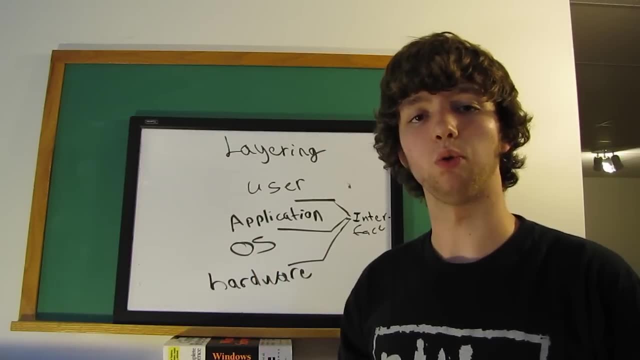 All right. so let's say I wanted to develop an application for a computer. I wanted it to be anti-virus protection, for example. So let's say I wanted to develop an application for a computer. 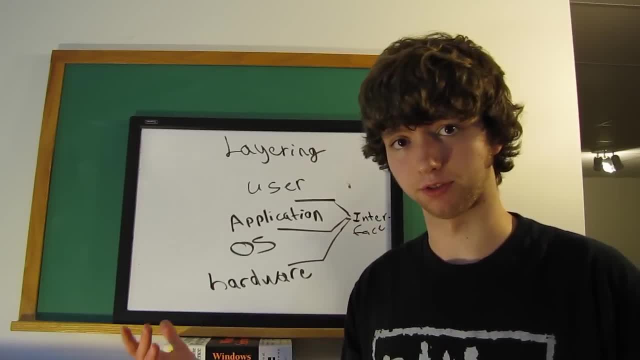 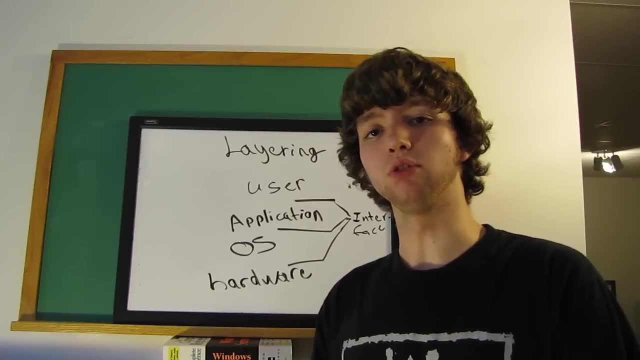 I wanted it to be anti-virus protection, for example. So that's just an example I could all right. well, let's figure out how I can do this. I can develop new hardware And then. 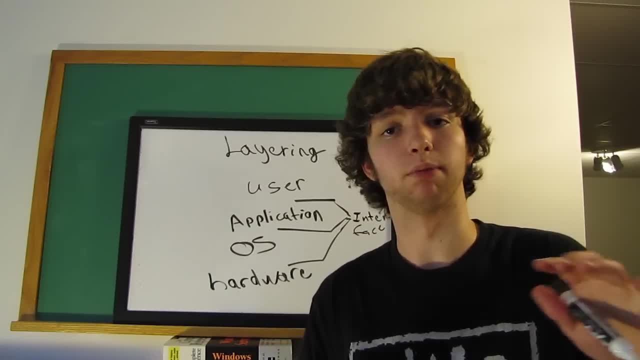 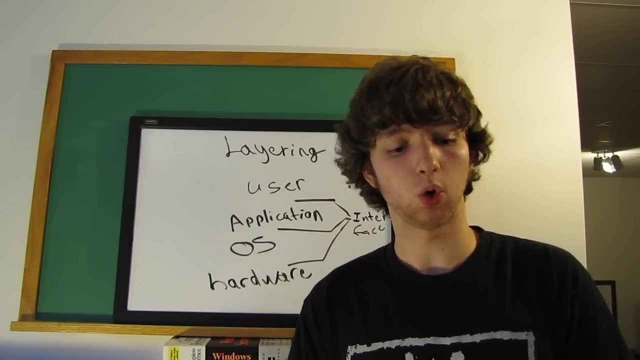 once I got that, I can develop an operating system And then I can develop the application. And, by the way, I'm going to develop my own programming language because I don't want to use anybody else's. 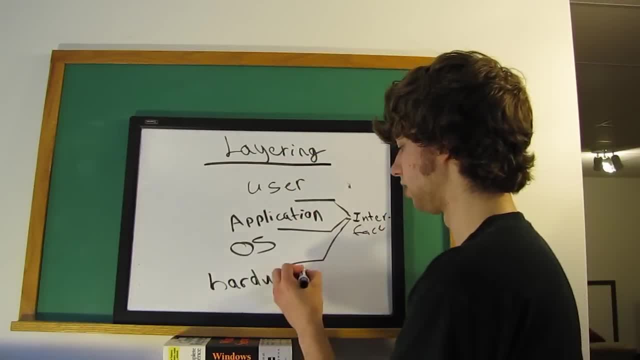 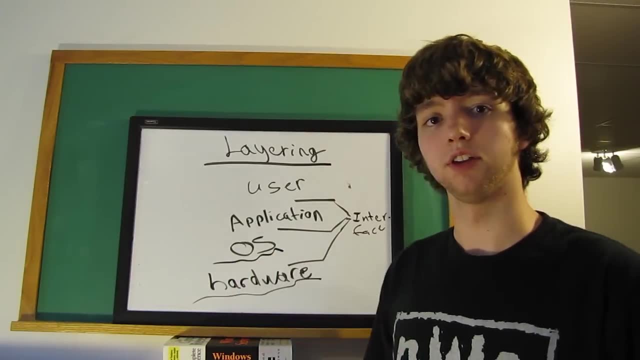 I can do all that by myself, Or I could use what's known as layering, Which allows us hardware is taken care of, operating systems taken care of. There's some programming languages I could use. I could use C. 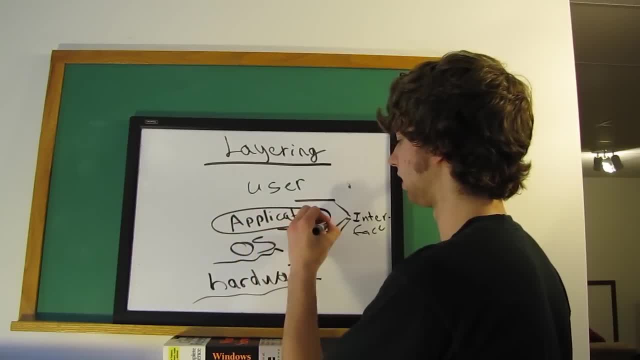 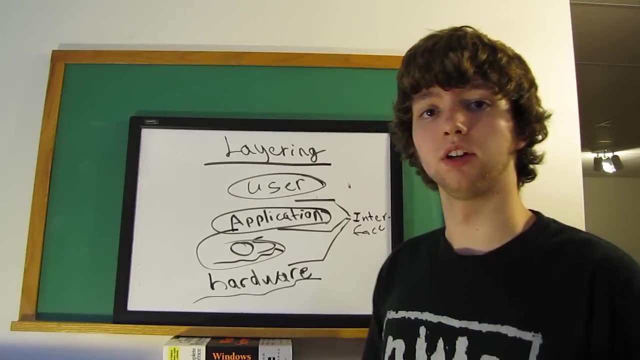 for example, And then all I have to do is worry about the application and how the application communicates with the user And how it communicates with the operating system. So that's an example of layering, where we look at everything. 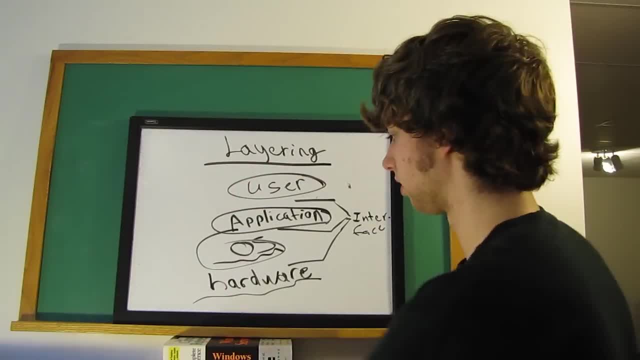 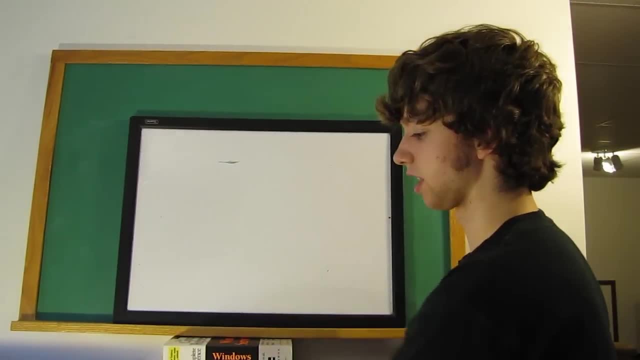 in a system of layers, So that way we don't have to look at it in a confusing manner to where you're not sure what's what, Rather than just saying, like computer, you could break computer up. 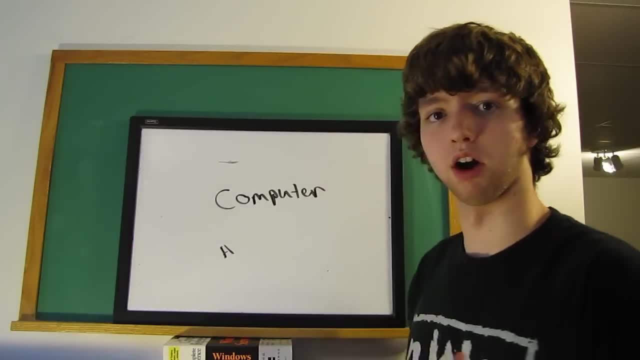 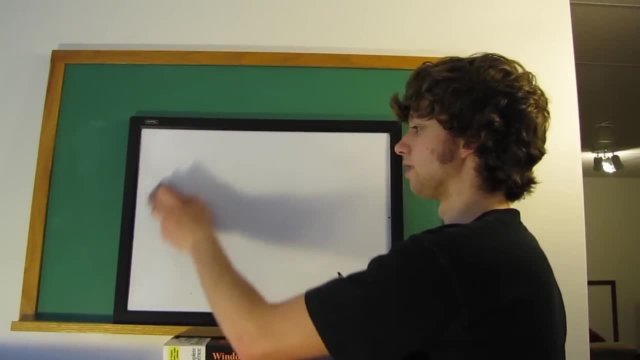 into hardware, software, operating system and the person using it. So that is the idea of layering. Now, to illustrate this very easily, we could, I'm gonna use alright, so let's say this: 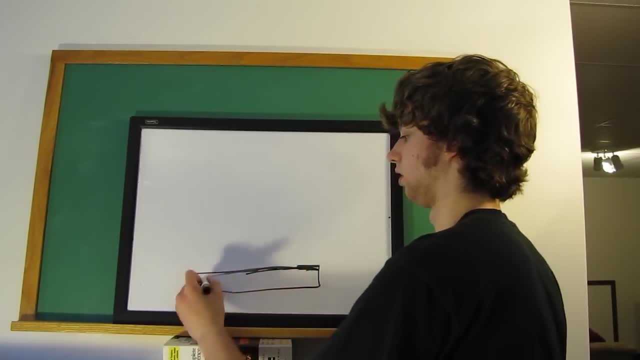 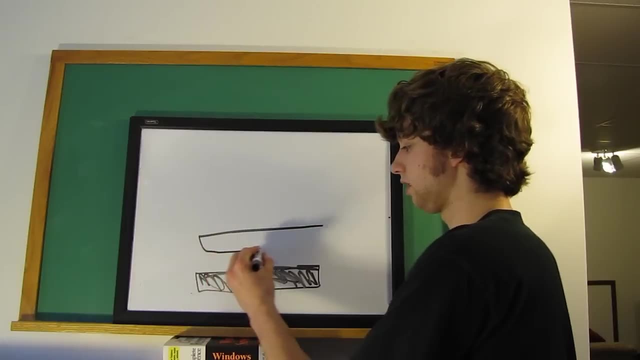 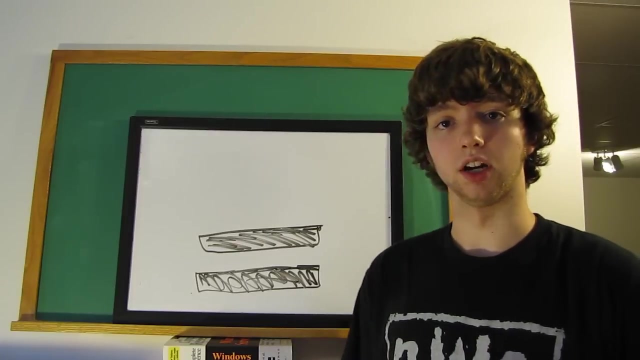 is the hardware, Alright. gonna try and fill this in real quick. And then this up here. this is the operating system, right, Alright. so now the the interface between these two. this allows them to communicate. 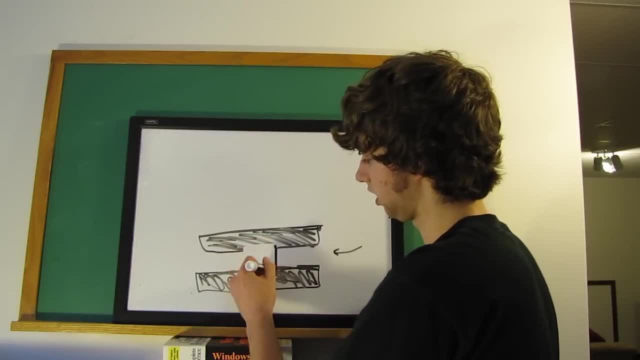 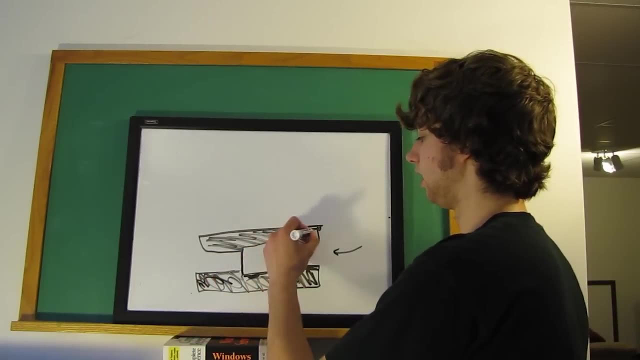 So we could say we have an interface right here Which overlaps a little bit, which allows it to take information from the hardware and use and give it to the operating system or vice versa. So this is the interface. 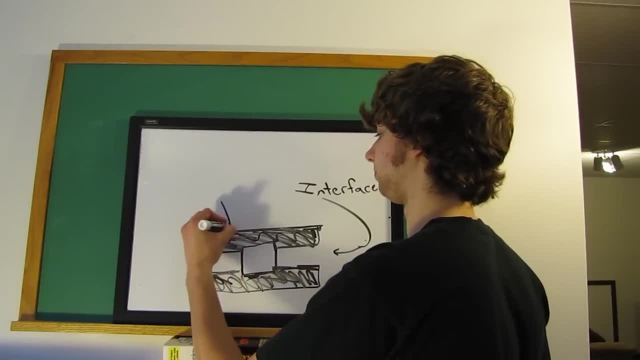 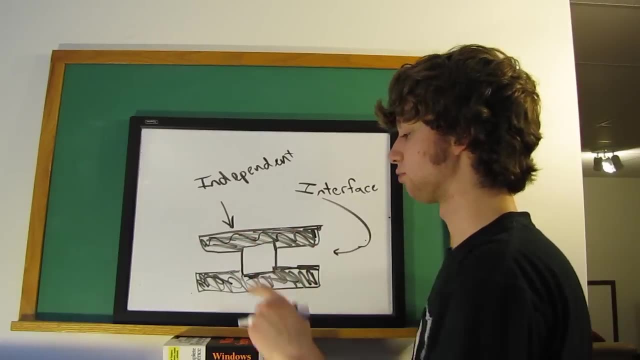 Now you could say these are independent. This is because they are different boxes. They are black to represent that this box doesn't know what's going on in this box. This box doesn't know. 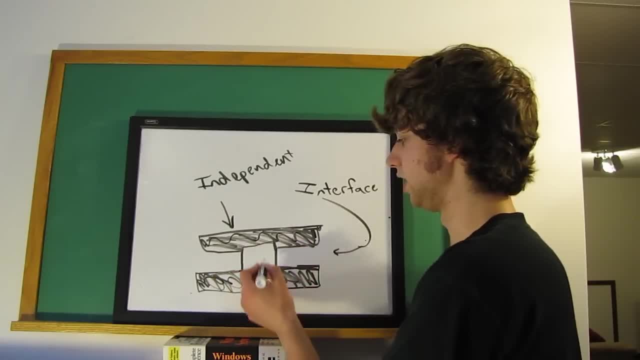 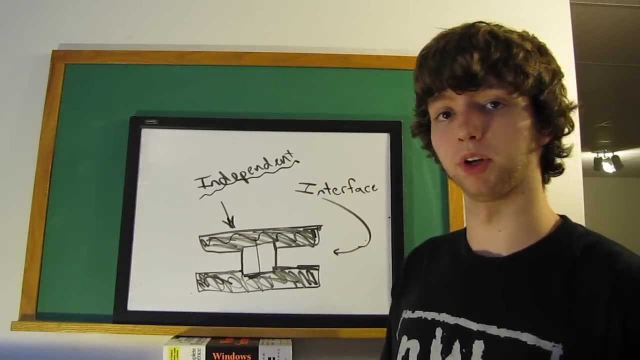 what's going on in this box. The only way they communicate is through the interface here, So that is to say they are independent. So when we are working with applications, so let's say we have another box here. 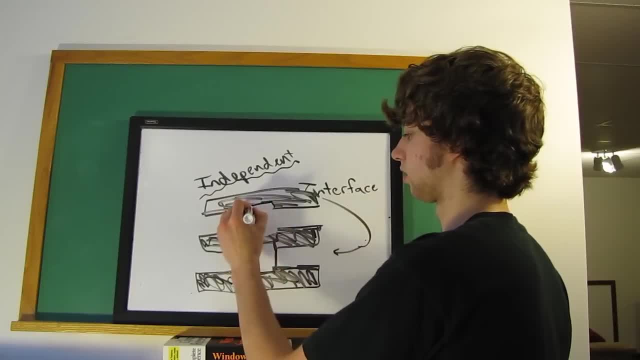 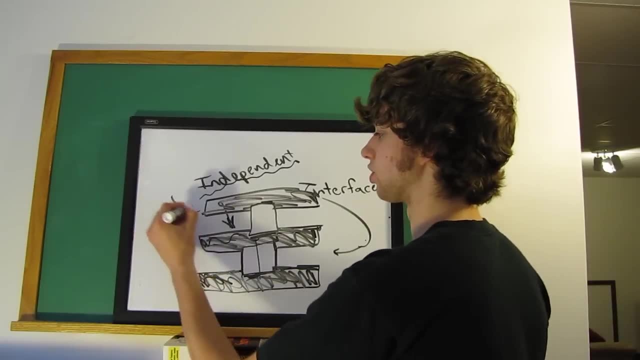 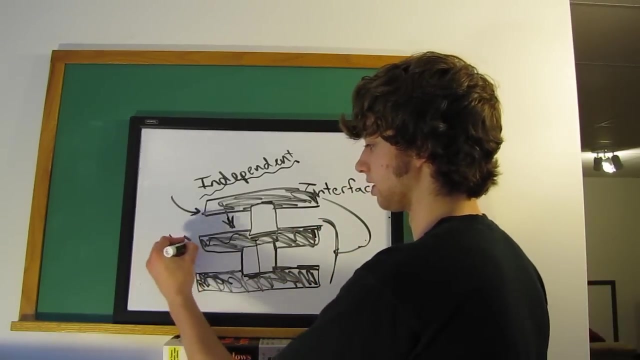 and then we have an interface between these two. Well, now we can basically change stuff within the application and it's not going to affect these other two layers. We could change something within the operating system. 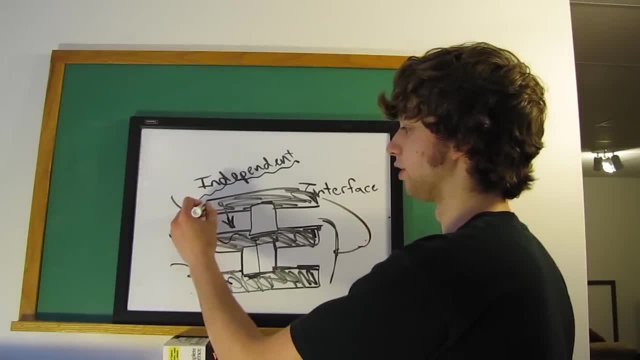 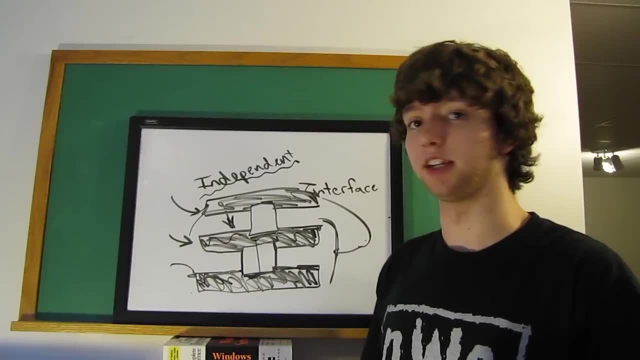 and it's not necessarily going to ruin these two layers. You could say they're independent because you can alter them. So, for example, I can update my Windows 7 computer and give it new features or whatever. Microsoft downloads for me at that specific time, and then all my applications should still work and all my hardware still works. The only thing that may change is the interface. So if something doesn't work, this interface. 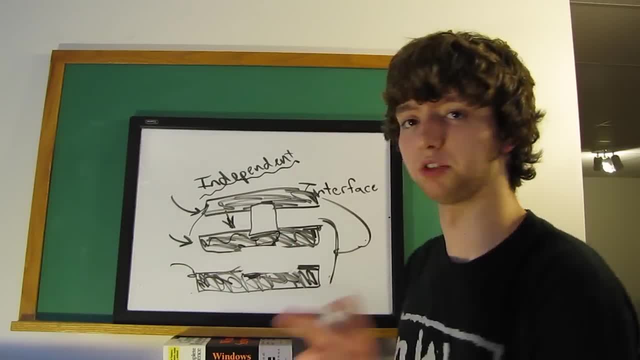 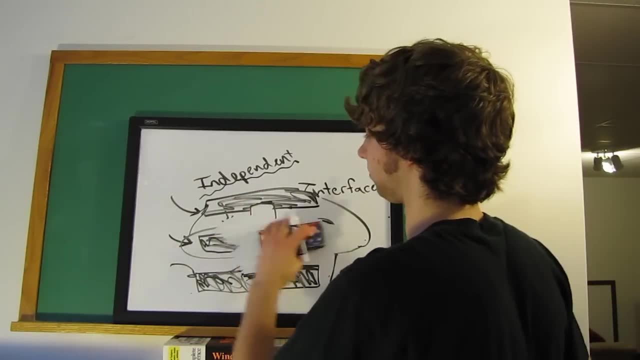 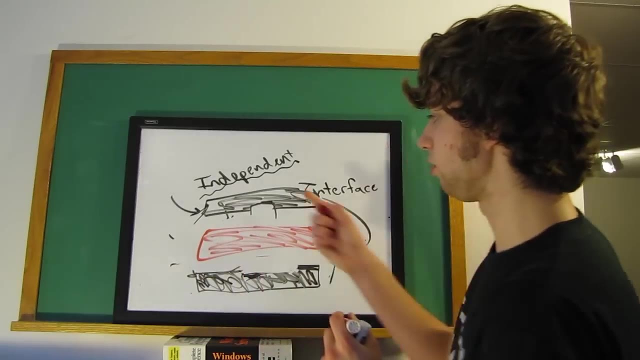 might have been destroyed or not working properly to allow them to communicate, But by changing this layer, since it's independent, I could change it, and now I have a red box, for example. Well, guess what? 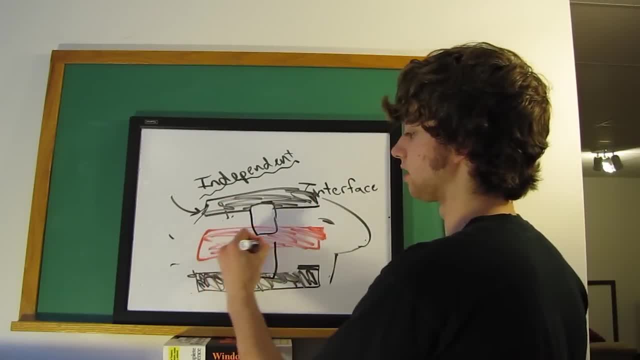 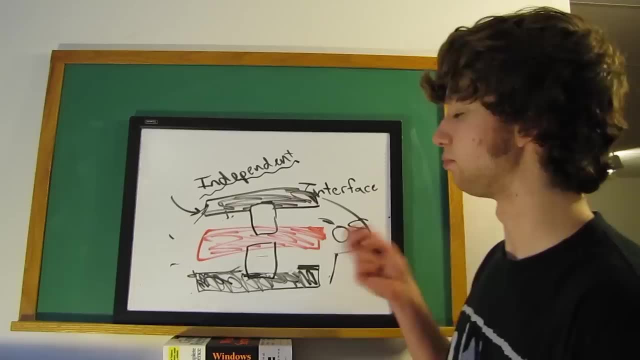 All these boxes are still black and the interfaces still exist. The only thing different now is my operating system. So that is to say, these boxes within the layer are independent, This system of layering. 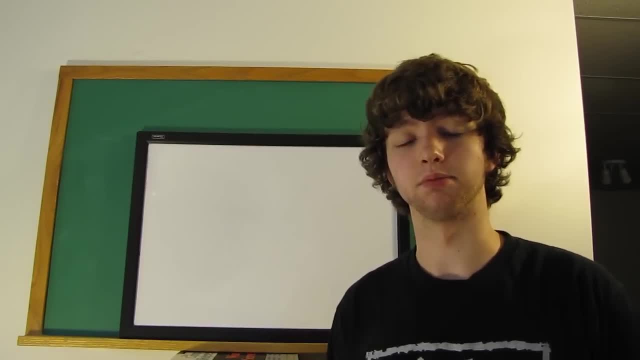 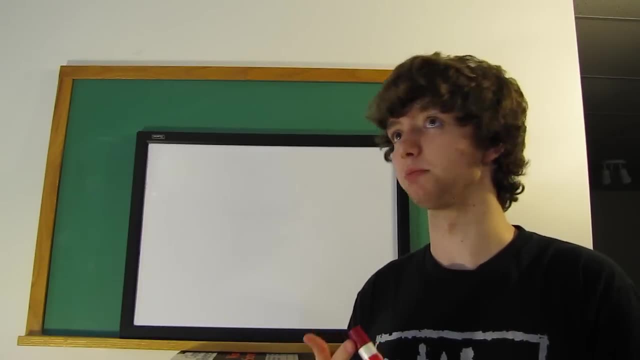 is also useful for computer repair and system design, because it allows us to figure out what's wrong with the system. It can either be part of the hardware. Is something wrong with the hardware? Do I need to replace? 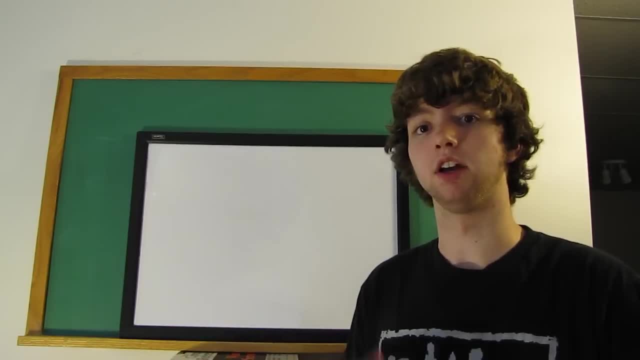 a processor, Which I mean probably not. Do I need to replace a hard drive? Do I need to replace a video card Or is it part of the operating system? Is something wrong with the system files? Do I need to reinstall? 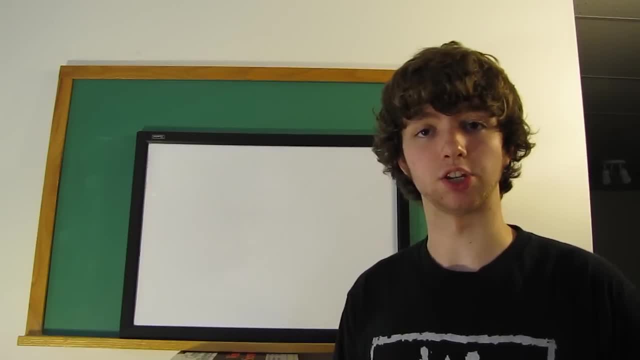 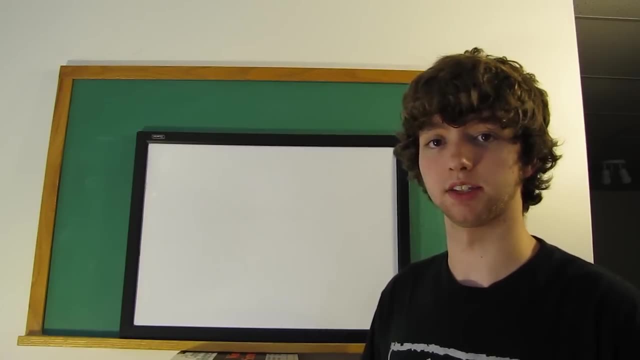 the operating system Or is something wrong with the application I'm using? Is there a bug? Do I need to download a software patch? This can help for that, As well as system design, because we can break up. 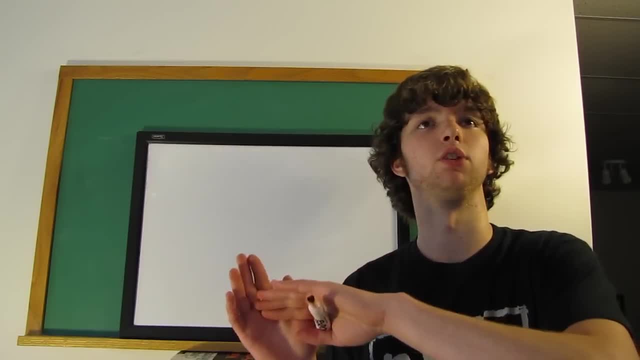 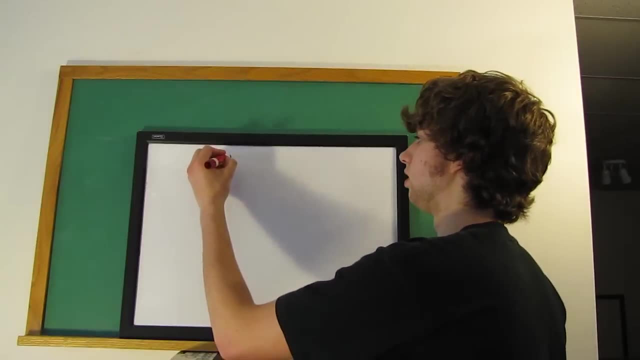 these specific groups which allows us to. we can, if we need to work on the operating system, we can ignore the hardware for a minute, We can ignore the application layer and we can just explode or enlarge. 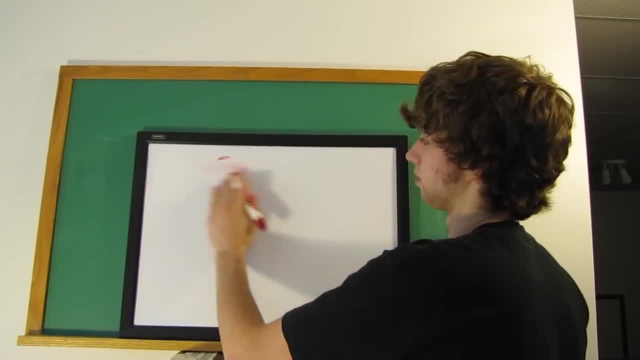 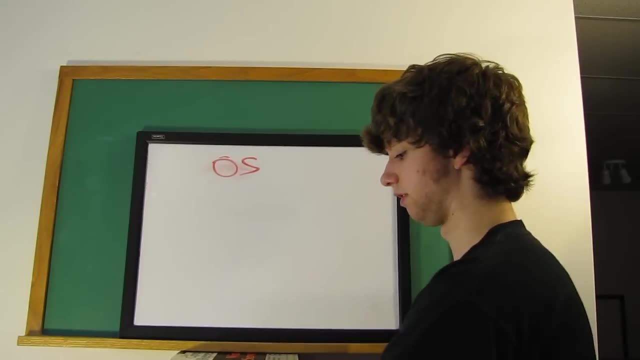 the operating system- Sorry, OS, because I'm lazy- And we can see all the different things that the operating system has to do for the specific application. So the operating system does quite a lot. So 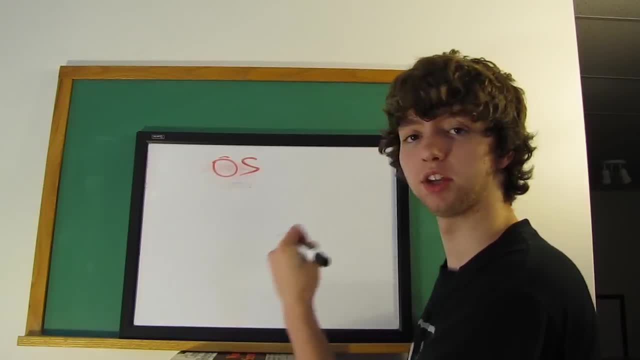 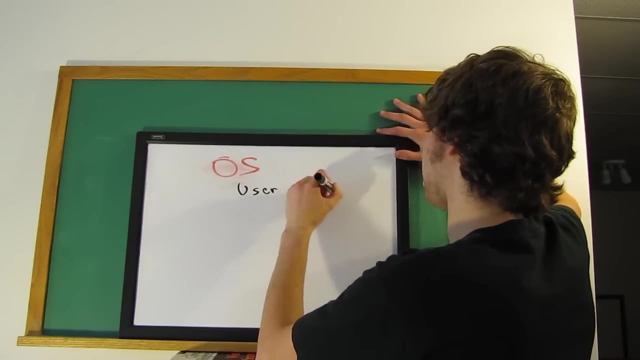 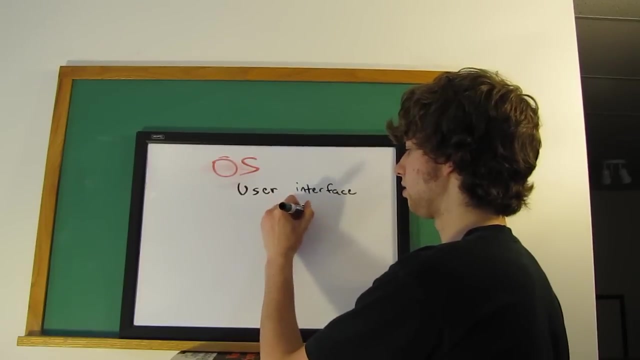 within the application, the operation, within the operating system, we have the user interface. So that is how we interact with the computer, whether if it's a graphical user interface- or you may see GUI, or if it's a. 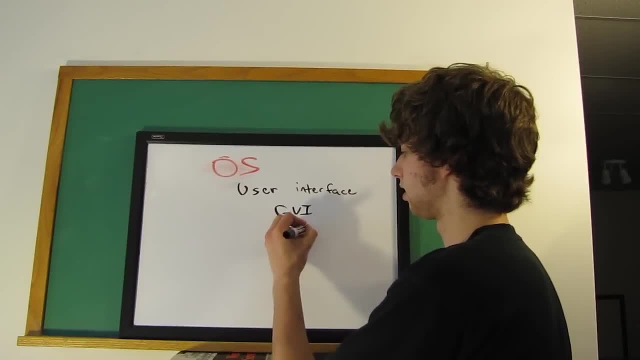 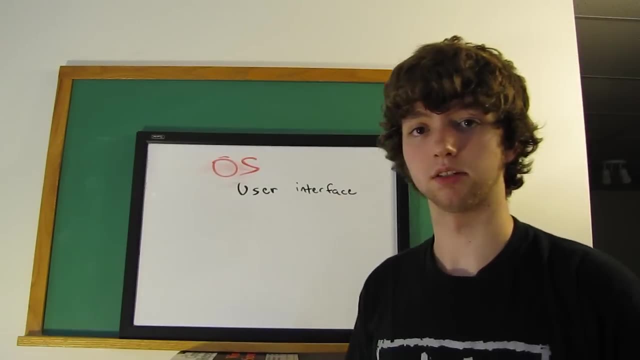 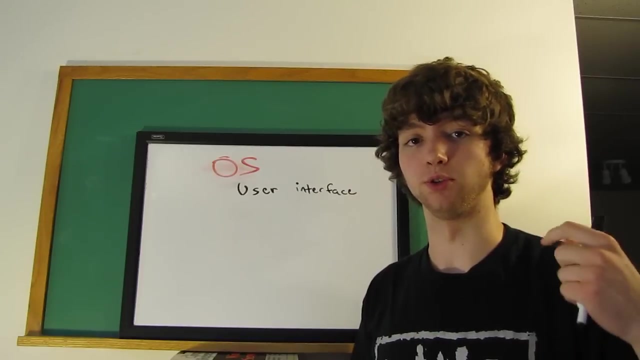 text, it can be a command line interface, But basically this is how we communicate with the operating system. So our visual, our as a user, we can use an application which then communicates to the operating system. 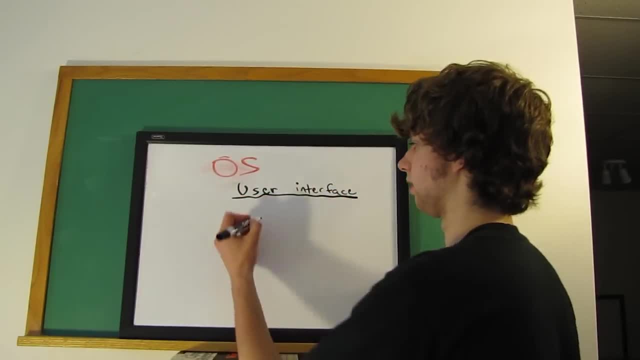 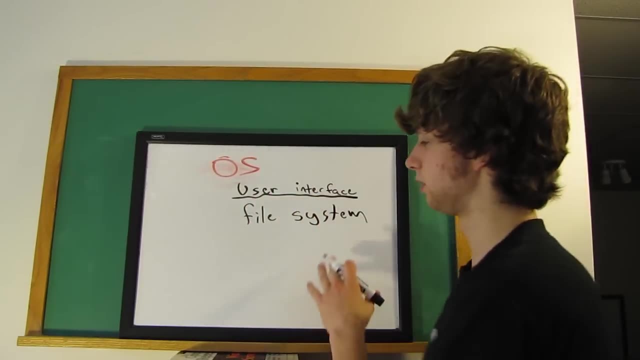 through the user interface which can then ask, then can affect the file system, which is the files on our computer. This, this system, allows us to open, edit or save or delete any files within. 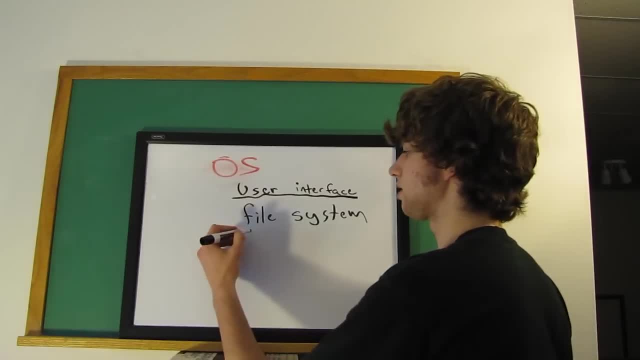 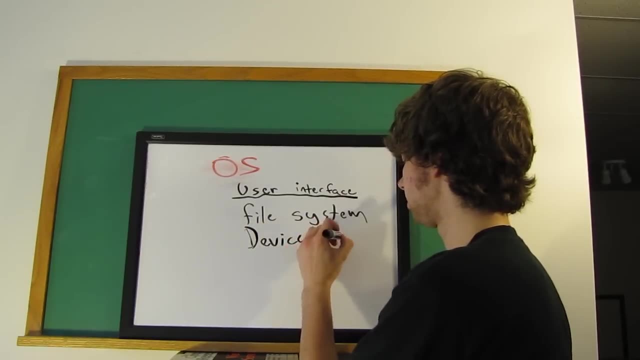 our system So we can also have device management. So this is going to communicate our peripherals- which peripheral is, I'll get to that in a second. Peripheral is something you connect to a computer. 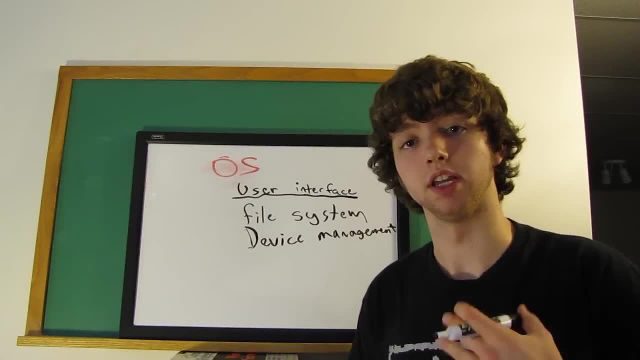 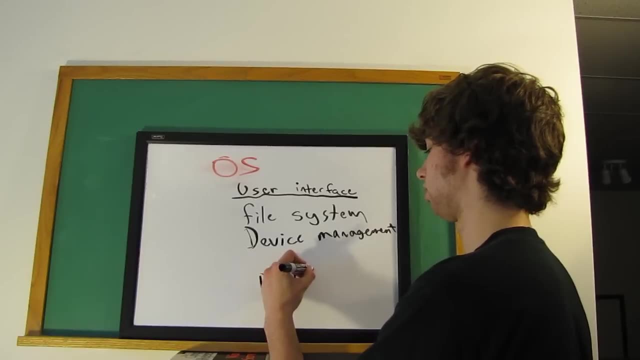 such as a printer, a monitor, a mouse, a keyboard and so forth. These are all known as peripherals. I don't know how to spell it, but I'll give it a shot: P-R-I-P-H, something like that. 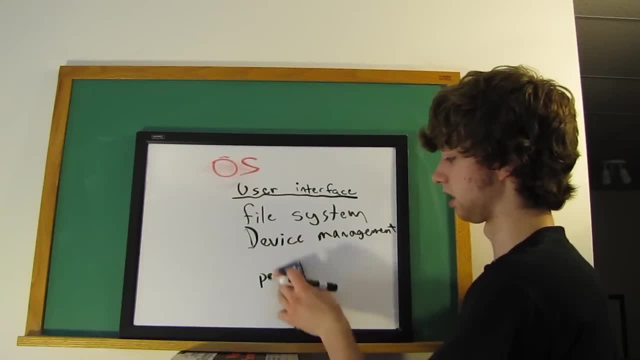 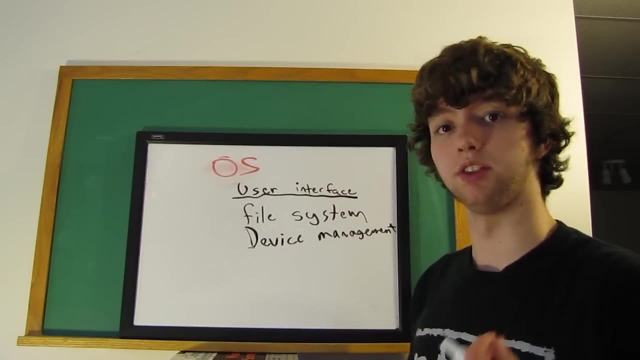 Don't take that for a. I'm- just just in case you couldn't understand what I was saying- Peripheral. And then there's also, like a, we could have the process management. So this is going to allow us. 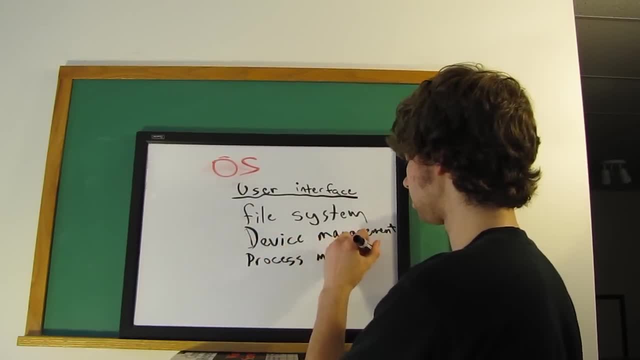 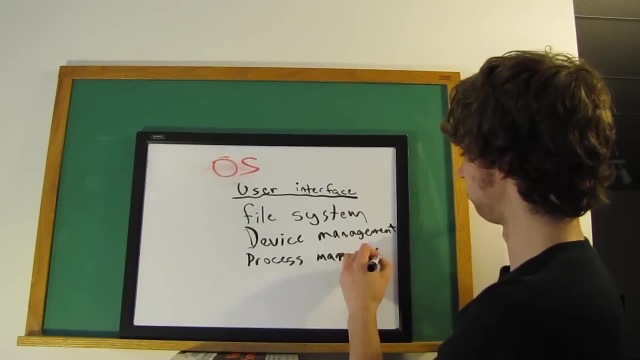 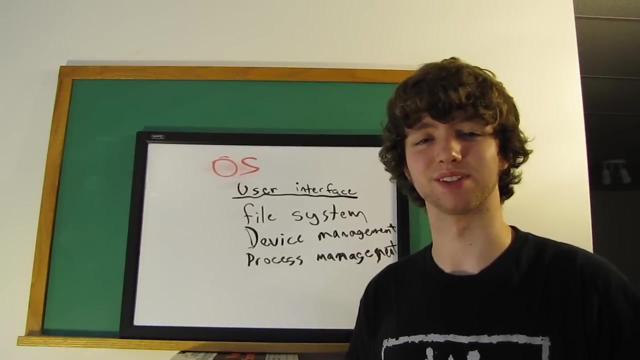 to run multiple processes which otherwise would be impossible without the operating system. So this I mean, unless we're programming, process management. So this is going to process the, the processes, process the processes, And it's going to allow us. 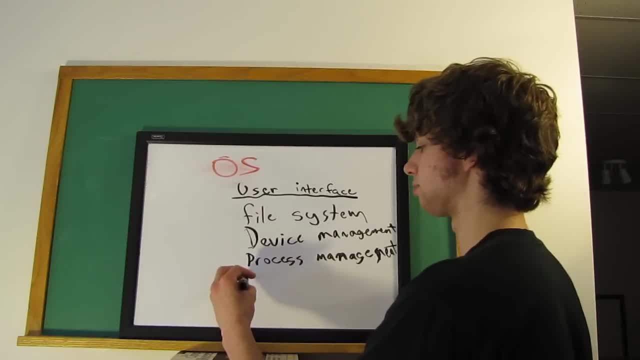 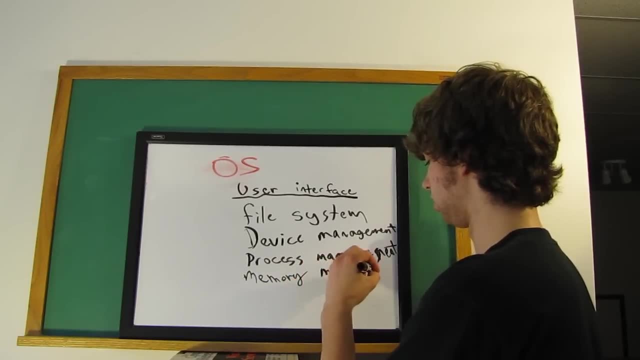 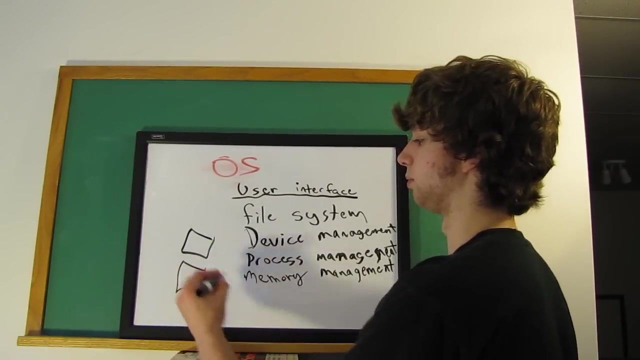 to run programs on our computer to have the memory management Which this is going to allow certain programs to use memory. So if we have memory multiple programs, it can share the memory within the operating system. 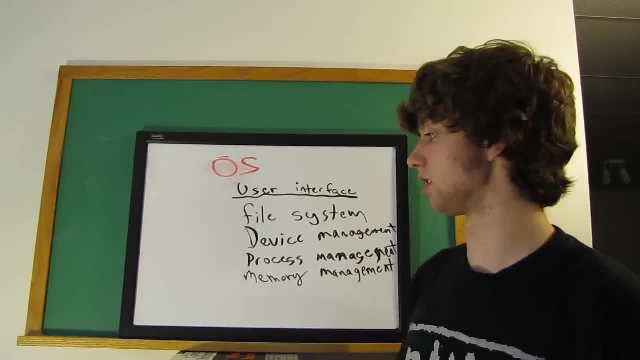 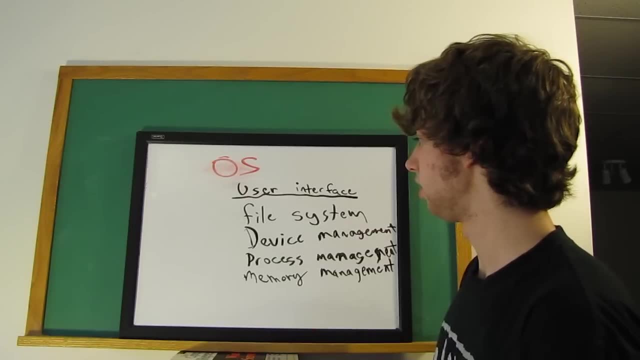 So this one gets a little, and then this one gets a little, And it also doesn't allow one application to override another application's memory in certain situations. So we have memory management. We could also have communication management. 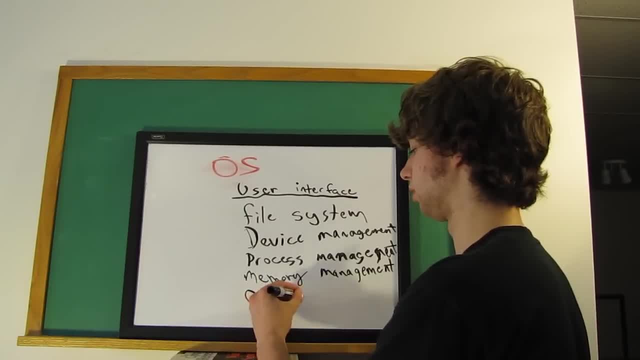 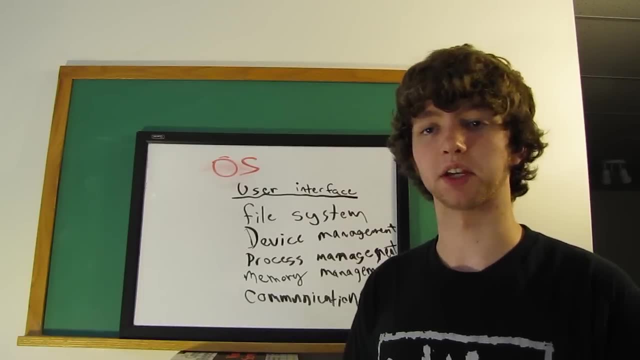 Which allows us to communicate with other computers. So if, if both operating systems have a means to communicate, then that can be done through the operating system. So these are just some examples of things that are on the operating system. 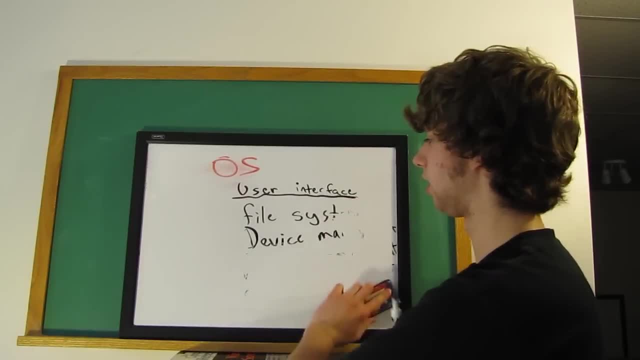 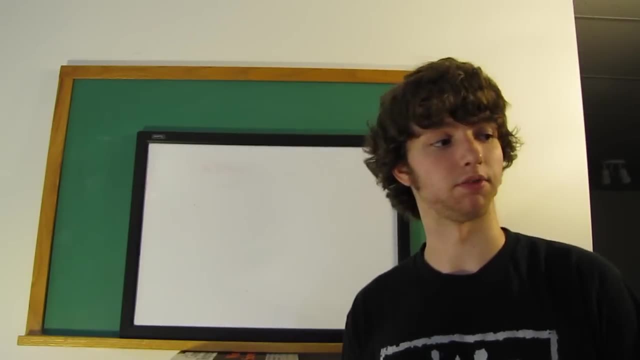 And if we didn't have an operating system, we would have to figure out how to do that within the application. There's a couple problems with that because obviously we'd have to change which hardware we're talking. 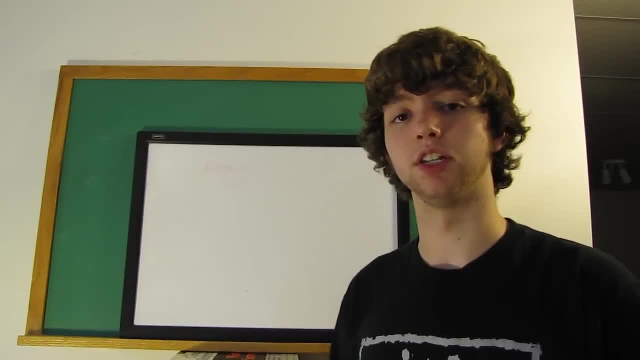 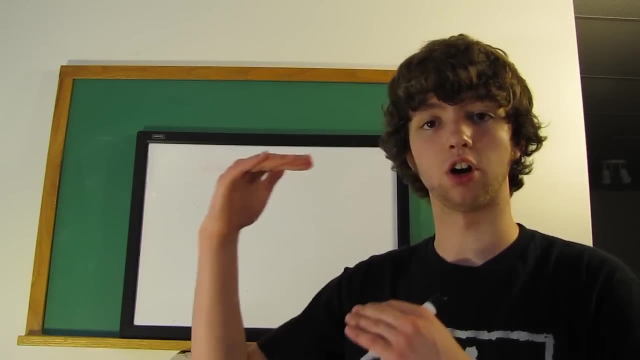 And also it would get a lot of redundant information, because if every single program had to do this, it would be a lot of extra content for each program In order for it to run. So the location of the 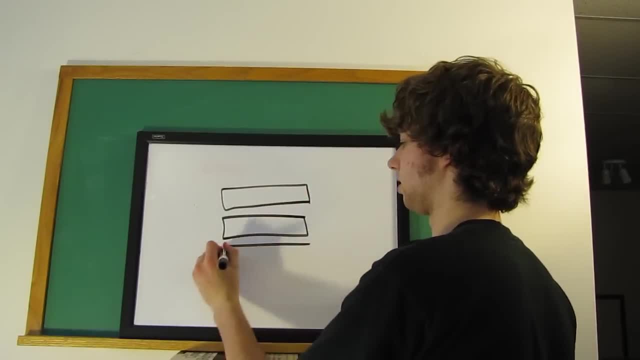 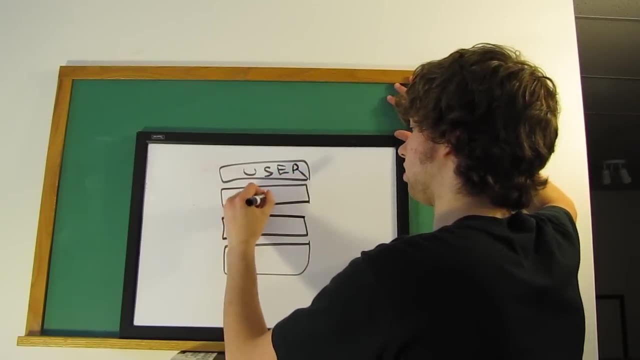 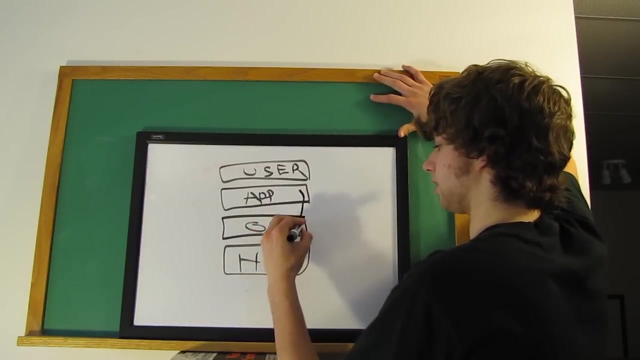 operating system in the layers. So we have the user, the application, the operating system and the hardware. Well, the application has to go through the operating system in order to get to the hardware through the appropriate interfaces. 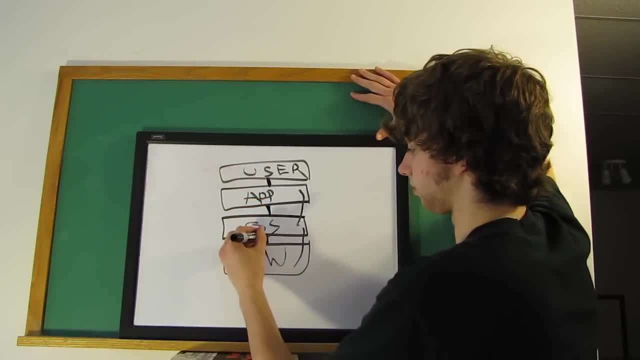 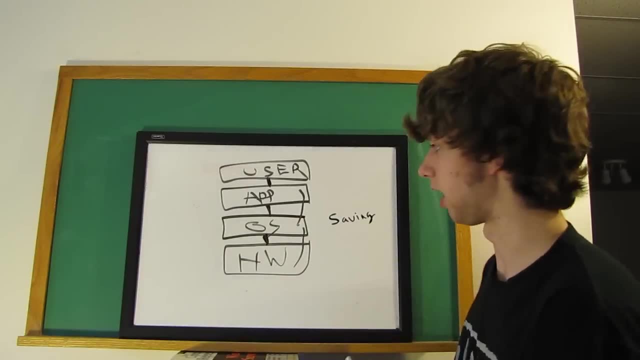 So if we have something such as saving a file or deleting a file, we can store that on the operating system and it's in the perfect location, because we use the operating system to contact the hardware. 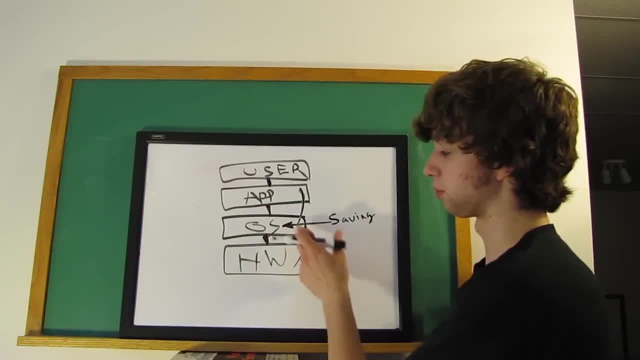 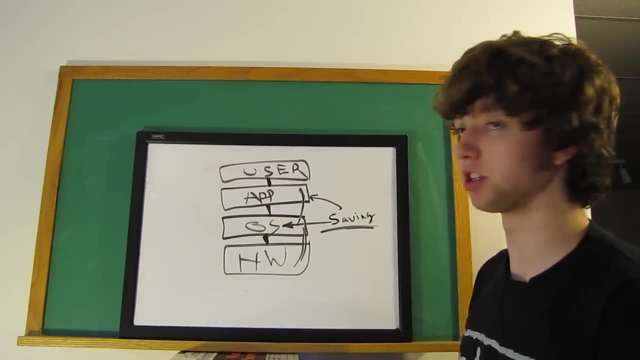 rather than having this kind of stuff stored within the application, It's great to have it within the hardware. So when you have a program and you can go to the software, and you can go to the software. 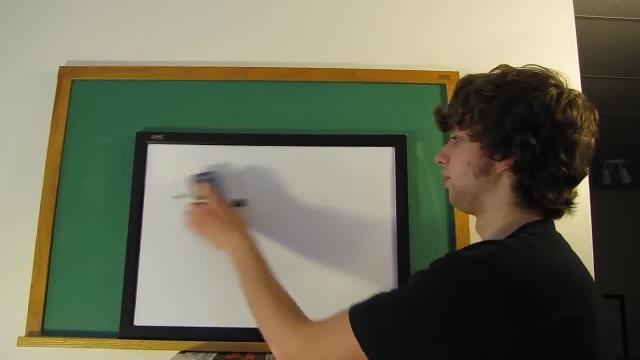 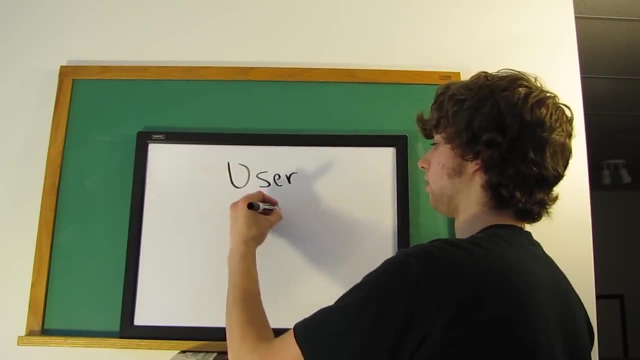 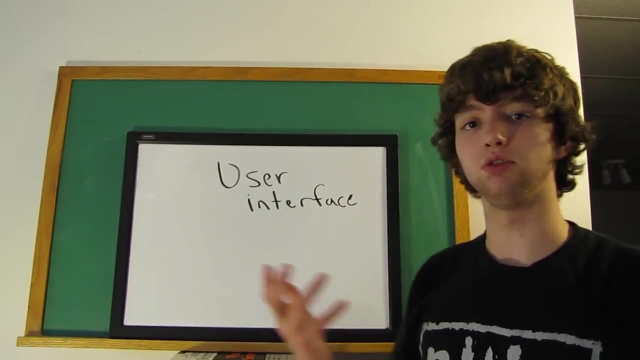 and you can go to the software and you can go to like file save. well, that's the user interface. Ah, this thing is so annoying Interface and this is going to do all this stuff within the operating system. 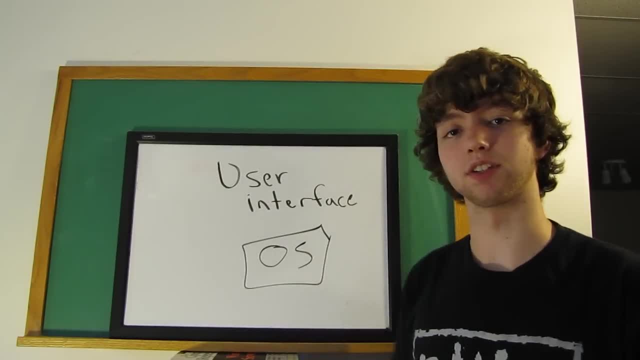 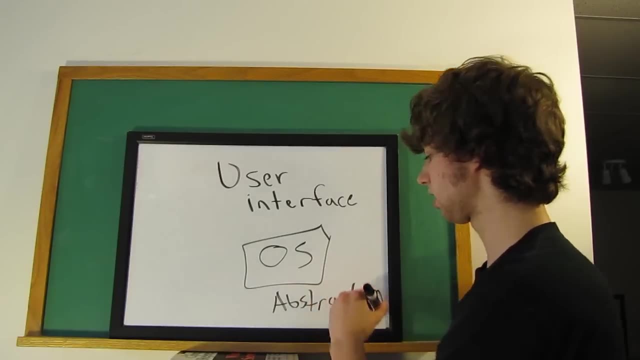 without necessarily telling us every single thing it does, and that's another example of abstraction. So just by clicking save or something, a lot of stuff is going to be done, a complex system, but all we had to do. 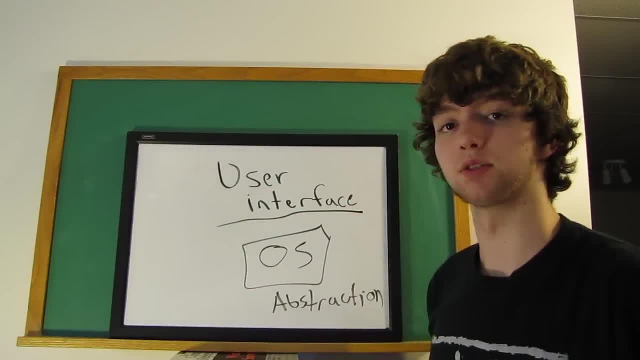 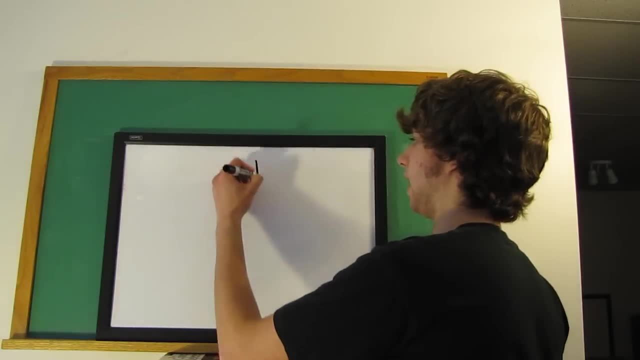 was click one button by the user interface. So those are some more examples. So there are many types of operating systems many of you have probably heard of. So, for example, we have the Mac operating system. 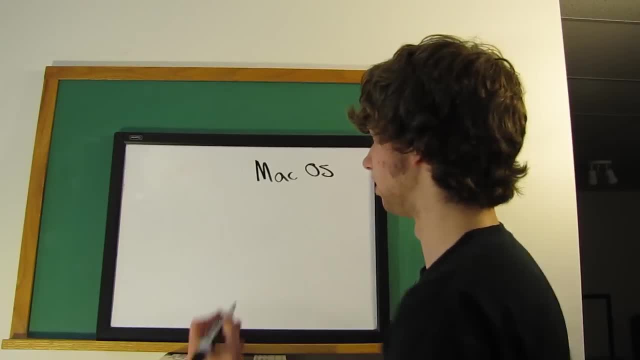 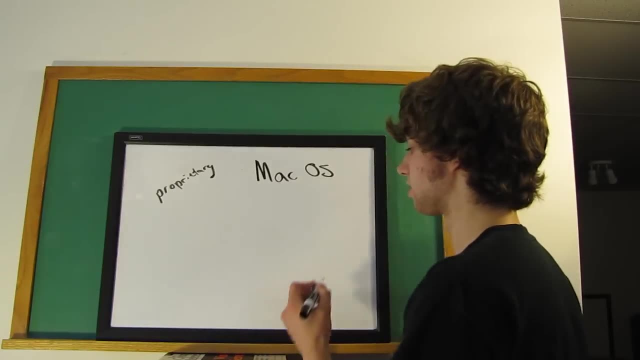 This is an example of a proprietary operating system. Basically, all of the Mac operating systems run on a Apple computer and they are not operating on a computer, So the Mac operating systems run on a Apple computer. 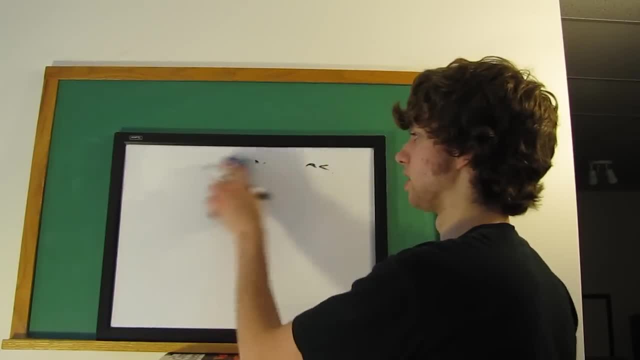 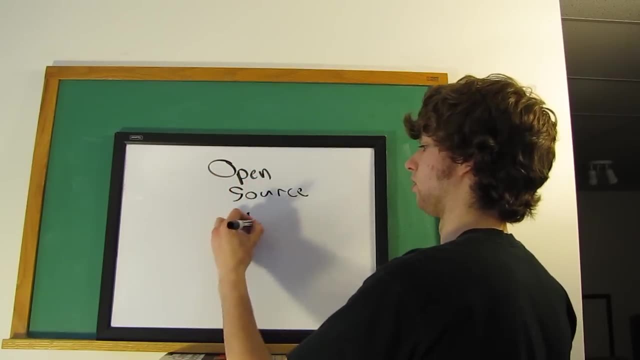 and they are not open source or anything We also can have, like, for example, Linux, which is said to be open source. This is an example of an open source operating system which displays its code publicly. 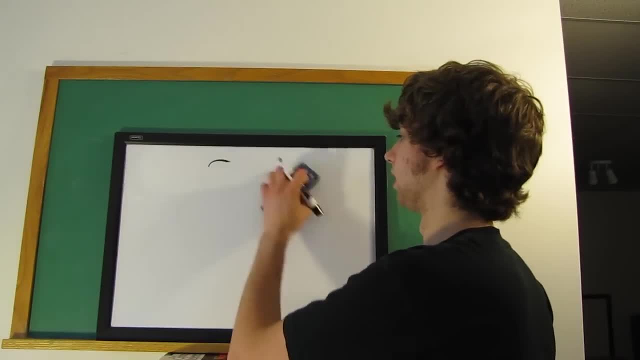 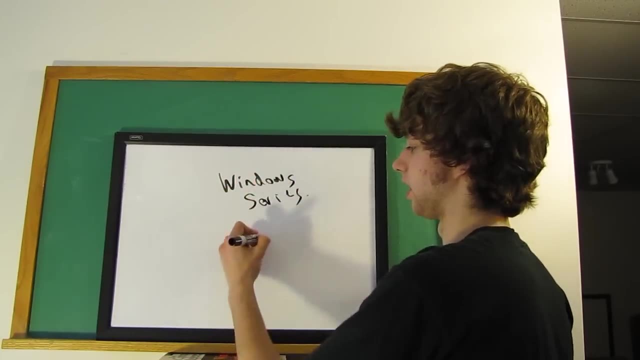 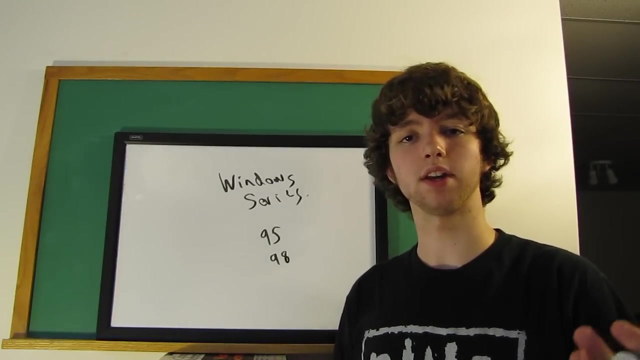 for people to edit and improve. Then we have like the Windows series, So like Windows 95, or 98, or 2000, and Windows 8.. Guys, I don't understand. why did they go from? Windows 2000, all the way down to Windows 7.. That's like a downgrade of 19,993.. So I don't under. I've never understood that. but whatever, Microsoft, But yeah. 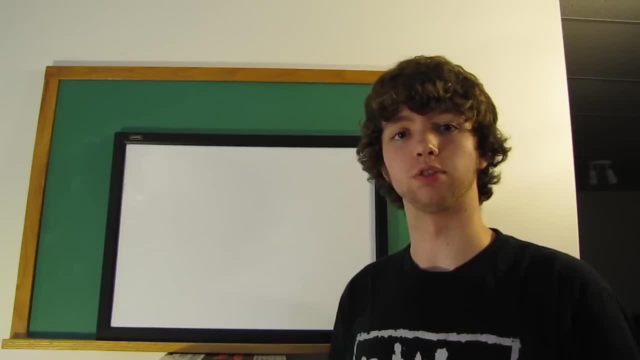 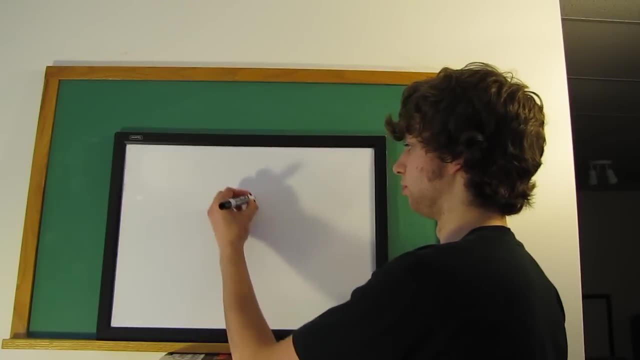 those are just examples. Microsoft is sort of in the middle, As in you can run Windows computer, Windows operating systems, on multiple manufacturer's computers, So for example Dell, Lenovo or Compaq or 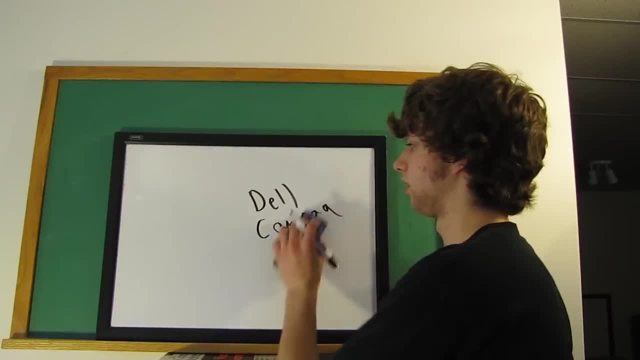 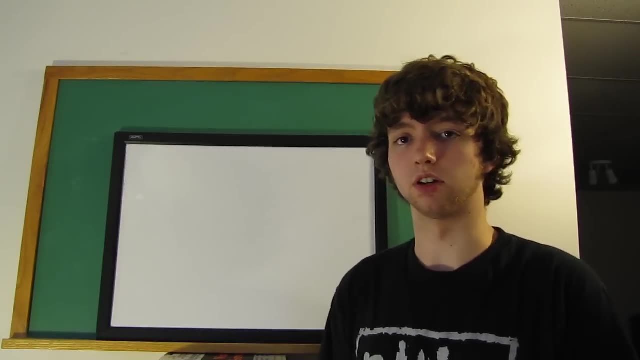 any any other computer brands- AMD and so forth. So, but it's not open source. So that those are some examples of some operating systems. That's pretty much all I have to say about operating systems. 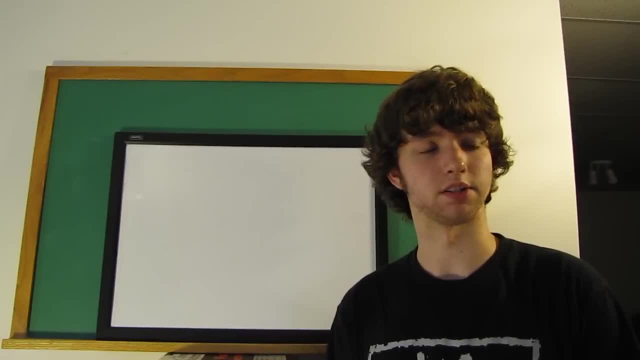 I'm gonna do a quick review And so if you guys don't wanna watch the review, that's cool, I'm cool with that. So thank you for watching. Be sure to subscribe and I'll see you soon. 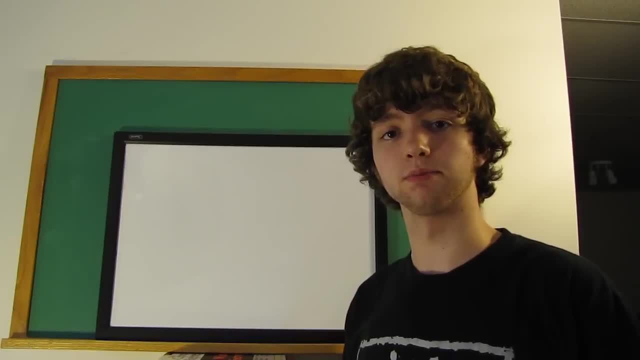 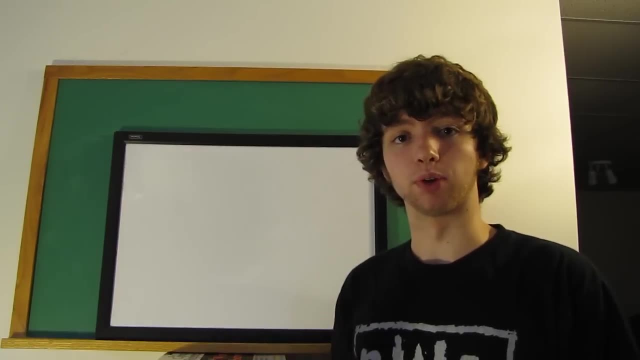 But if you're gonna stay, here's the review. Operating systems are a means to allow applications to communicate to the hardware more easily. The operating systems has tons of services which are basically miniature. 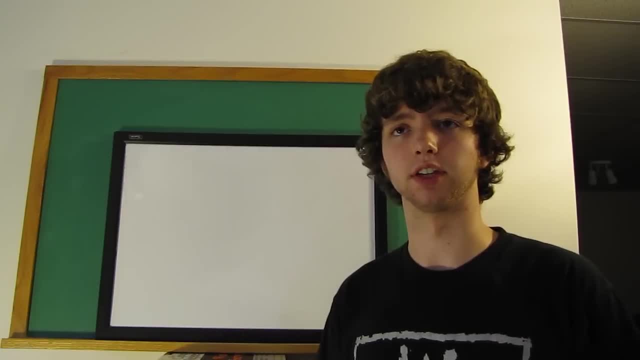 programs. I guess you can think of them at. I guess you can think of them as that. But basically services within the operating system include file systems management and so forth, which does certain things. So 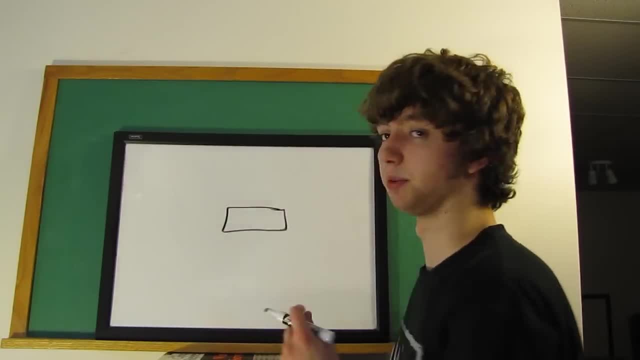 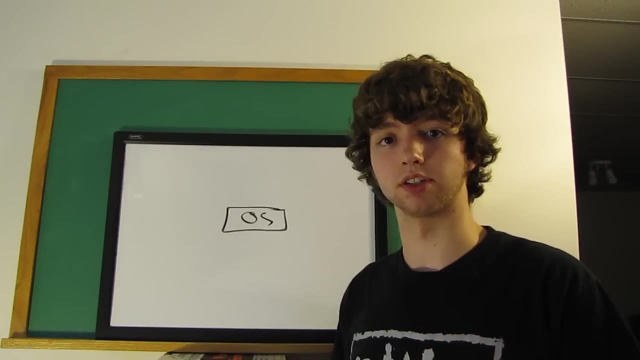 when we think of the operating system, we don't have to think of everything within it. we can just think of operating system We we don't have to think of the file systems and the communication systems and the. 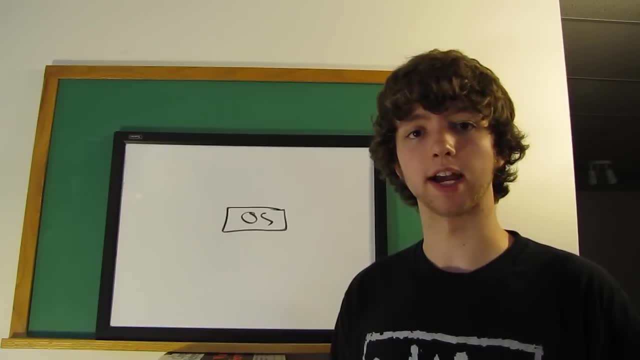 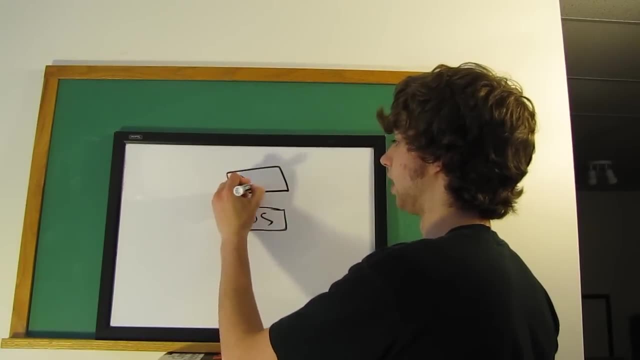 memory allocation systems. We can just use what's called an abstraction to make complex things very simple. So the operating system talks to the application. So, for example, the mail system and the operating system. 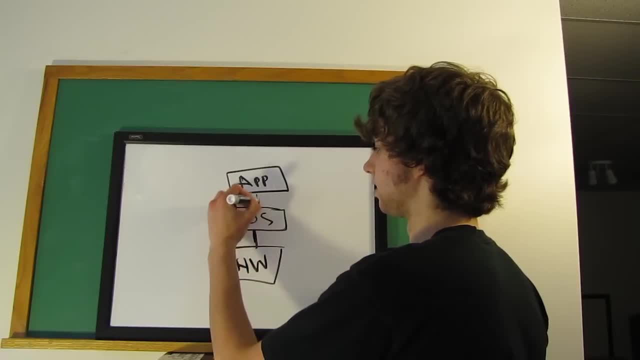 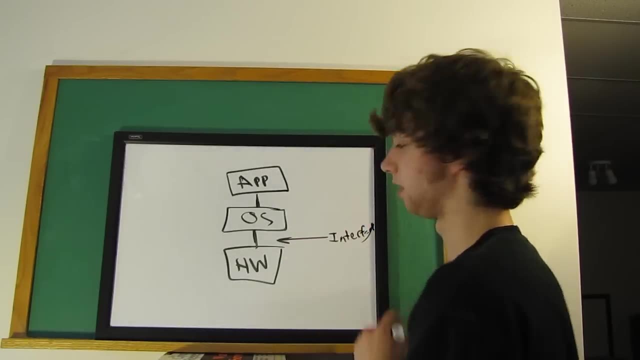 also talks to the hardware using what's known as an interface. So these right here are interfaces. I can't write anymore in that spot, but these right here are interfaces. and then the application is used. 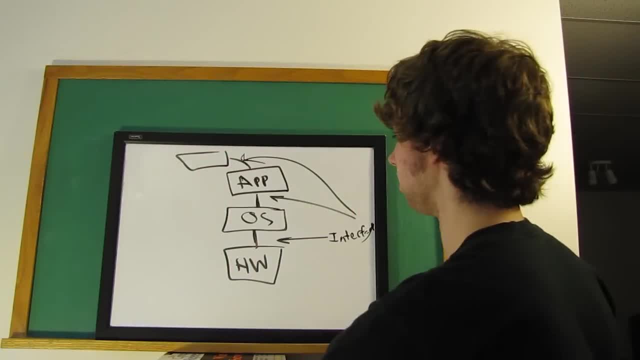 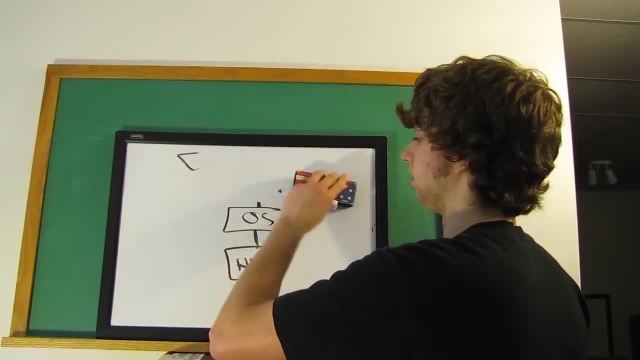 by the user, And you could say that's an interface as well. So the operating system allows us to easily use the hardware, and you could say that the operating system and the hardware together is what's known as. 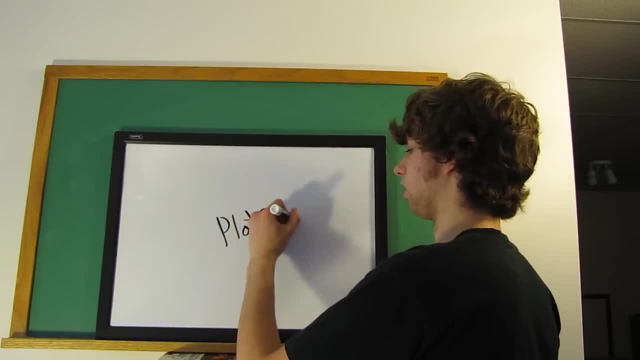 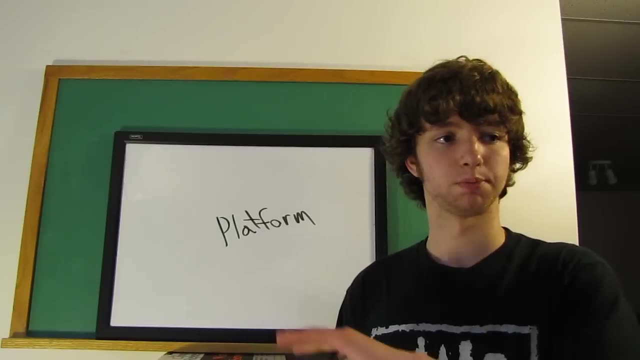 a platform which allows us or which allows app developers to easily create content for computers rather than having to worry about specific hardware and so much other garbage. So what we can do is we can think of. 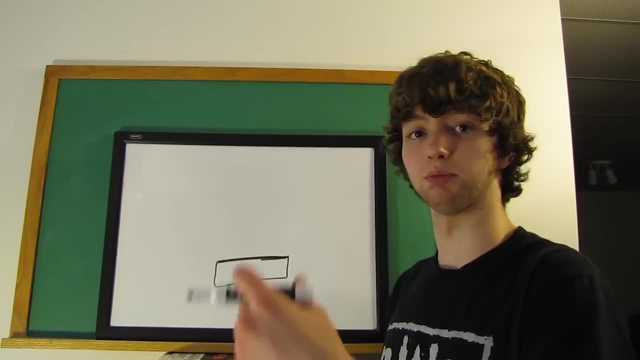 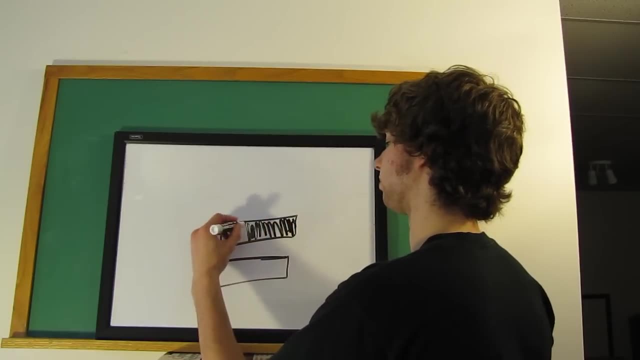 a layer within our layering system. Layering system just breaks it up into these individual abstractions. We can think of these as unique and isolated boxes, that this box doesn't know what's going on. 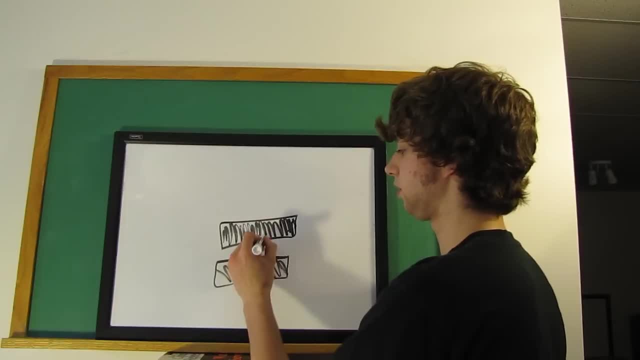 in this box. this box doesn't know what's going on in this box. The only way they communicate is through the interface. So that's, that's pretty much that, And then. so, basically, we can think of: 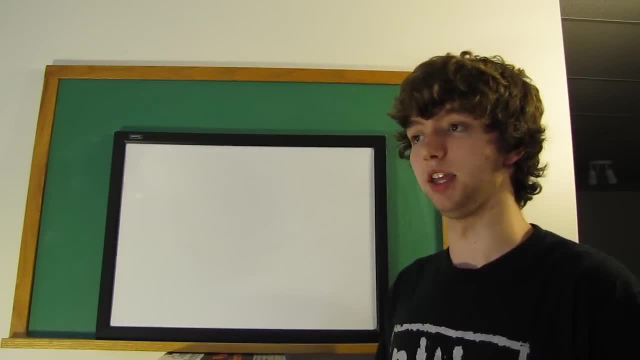 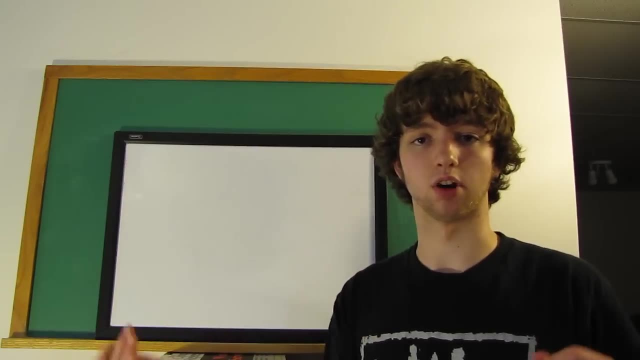 a specific layer within our layering system and we can enlarge that if we wish and get rid of the abstraction and think of the individual pieces within that layer. So let's say it's operating system. 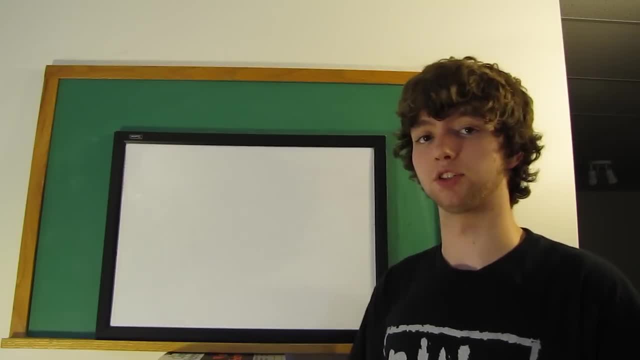 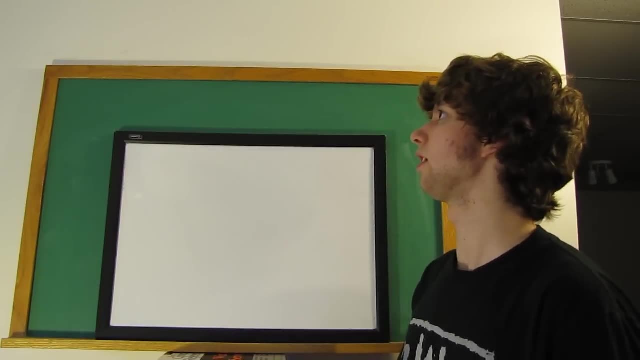 we can think about the filing system or the memory system and so forth like that, But otherwise you don't have to, So that's something we can do with that. And there's open source as well as proprietary. 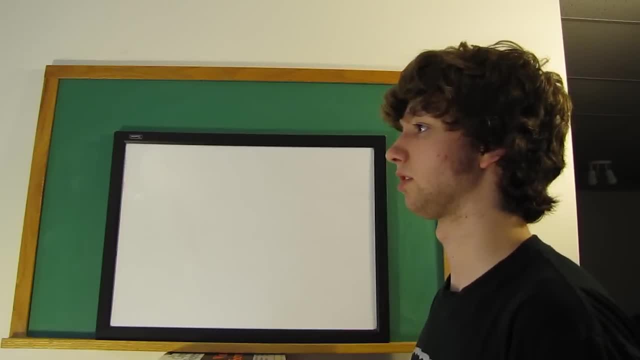 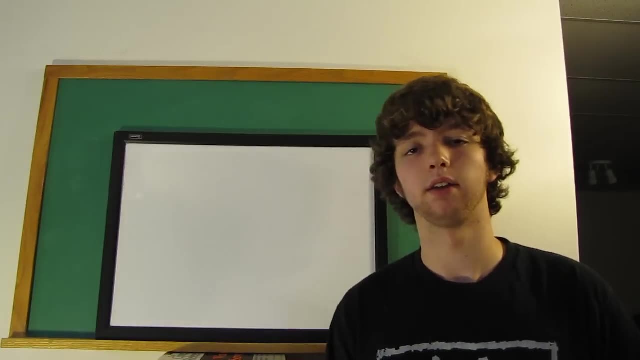 operating systems. What else did I talk about? I'm pretty sure that's about it, So I probably forgot something, but that's okay, because you can watch the entire video over and over again, So great. 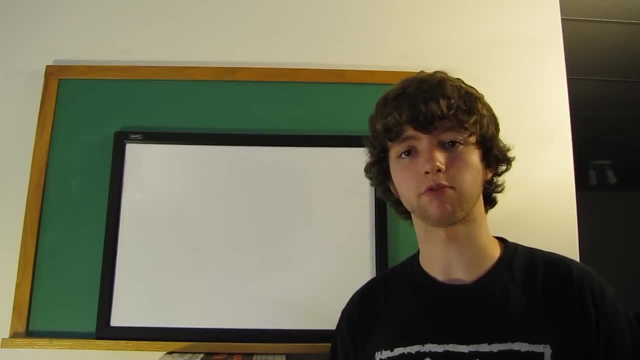 Thanks for watching. If you want to see some more stuff, be sure to subscribe to my YouTube channel. If you have any questions, please leave it in the comments below. Please tell me if any explanations are rough or what I need. 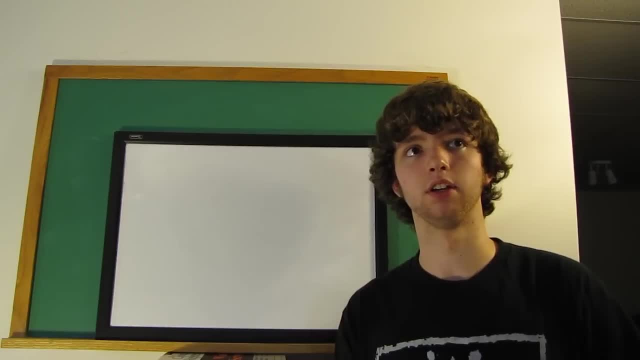 to improve upon, as well as how appropriate. I said this was a beginner's course. If it was too difficult or too easy, let me know and I will try to get a better rating system as I go. So thank you and subscribe.